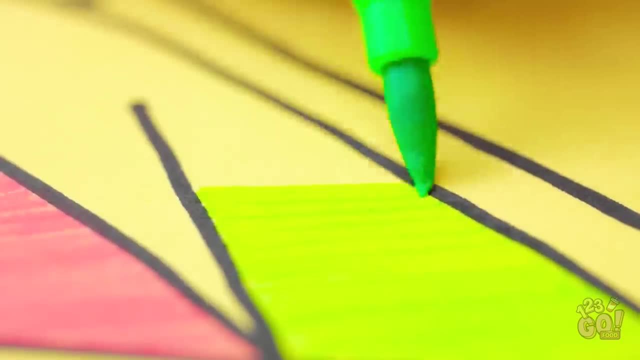 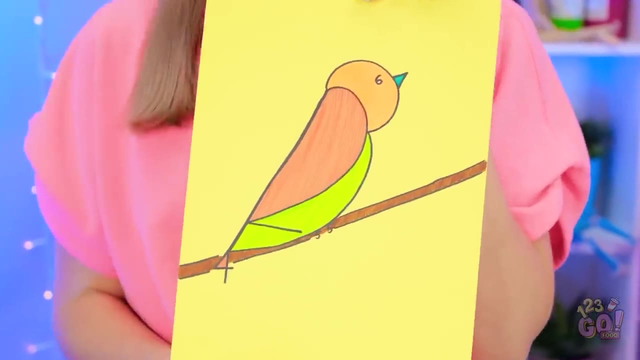 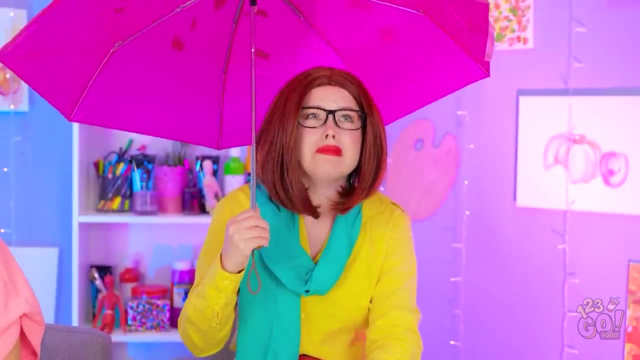 I'll give you nice beautiful feathers With all the colors of the rainbow. It's finished. What do you think? Can you see the numbers in it? Stunning. And you? I got stuck under some bad weather. This is as far as I got. 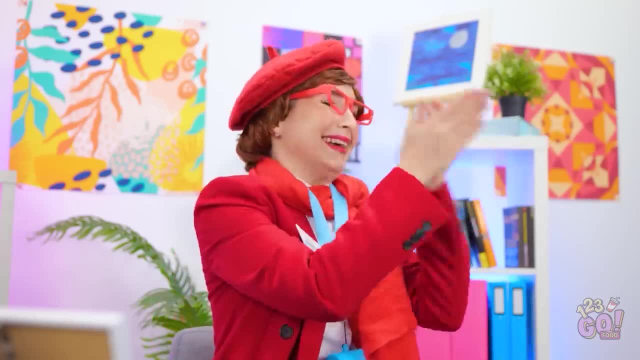 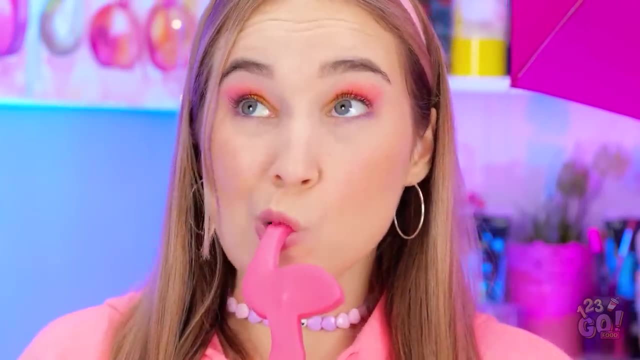 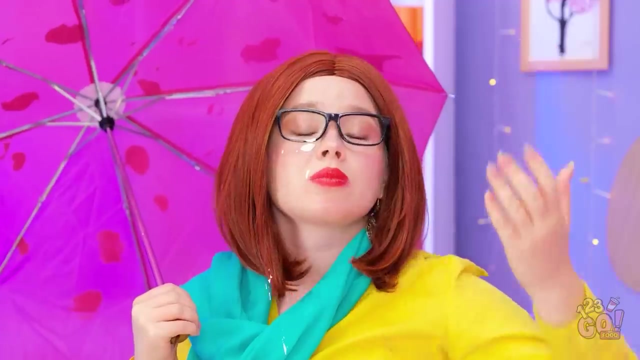 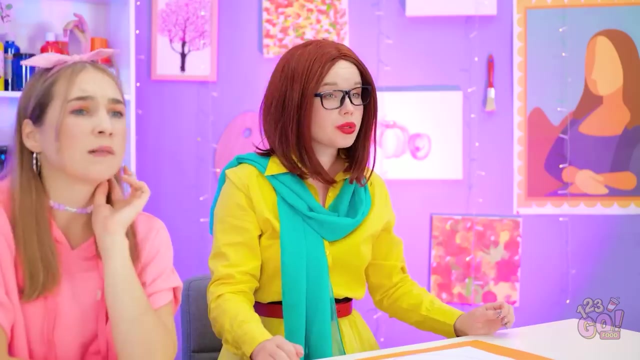 Ooh, You won this round, Annie. Aw, yay For me. Thanks. I can't work under these conditions. I guess I should've seen that coming. Oh, The next challenge is upon us. I've seen plenty of apples in my day. I know just where to start. 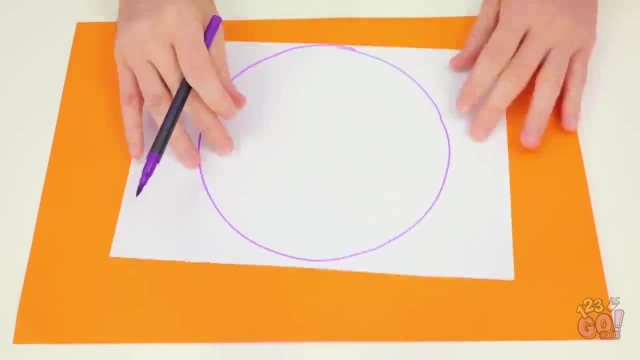 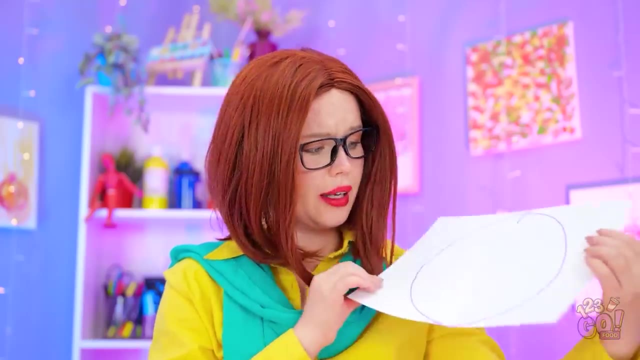 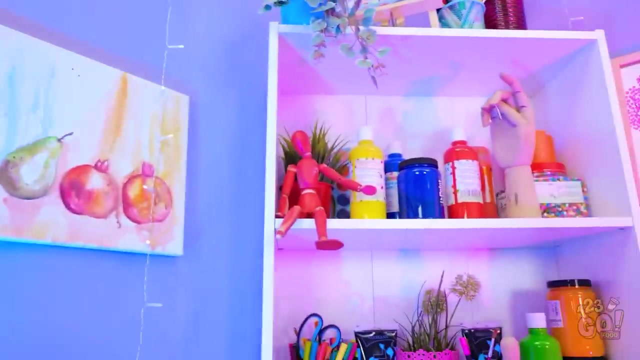 And the perfect circle is key here. But where am I supposed to put the stamp? This circle takes up the whole page. Ugh, Back to square one. Hmm, I could use a little inspo. Wait, I spy the perfect apple. 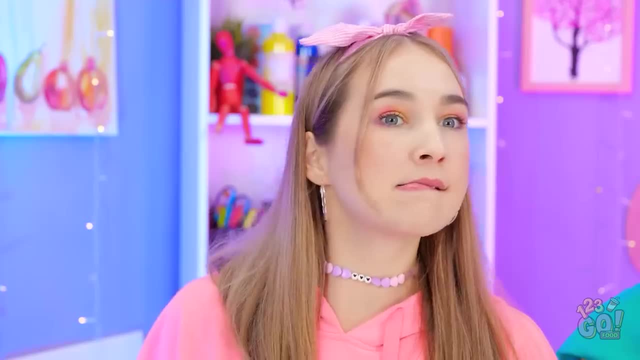 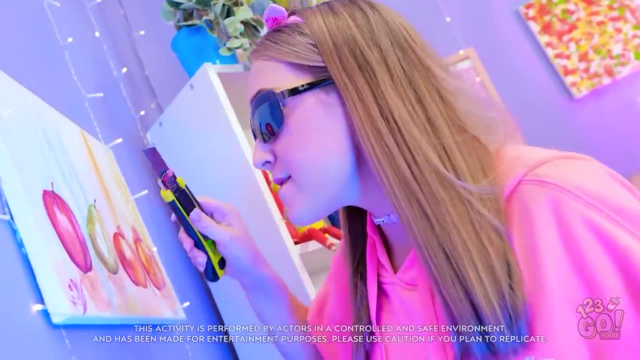 Mm-hmm, She seems good undistracted. I'm going in. Mission apple impossible in full effect. I'm armed and ready. A clean, careful cut is all it takes. Huh, What is Annie doing? Knock it off. 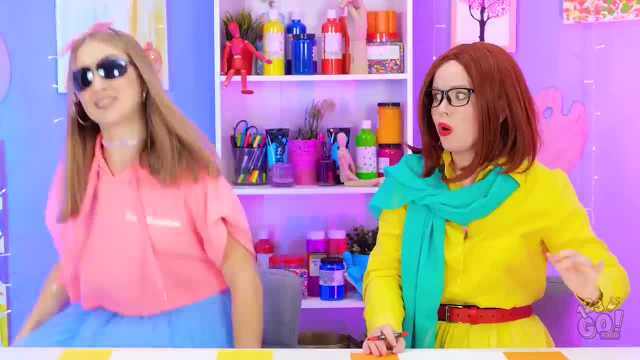 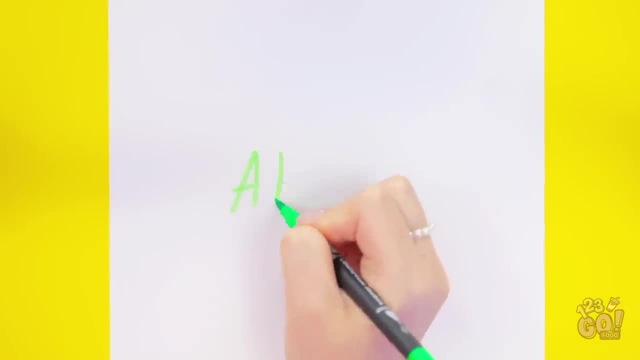 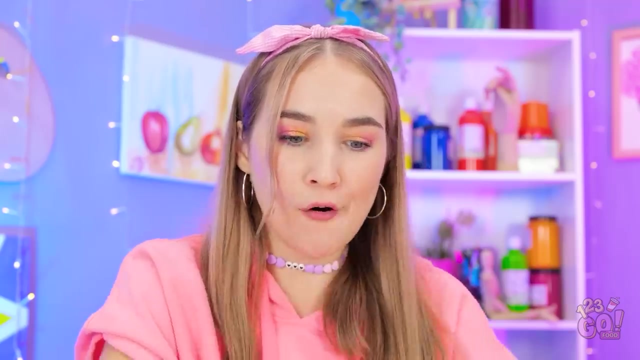 Sit down. Sorry, Aw man, I was close too. Hmm, Guess I'll just draw what I know, Like the word Apple, That's easy. P-P-L-E. Wait a minute If I divide the word by five. 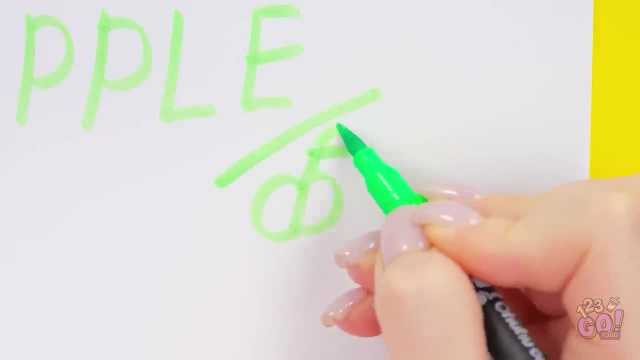 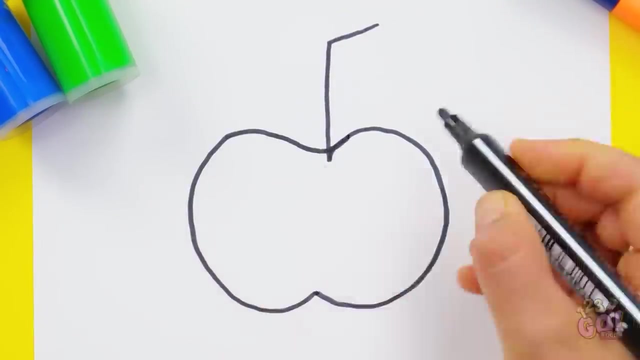 or rather an apple. I get one big step closer to my results. Okay, Let's make that five a little bigger. Who knew the number could take up a whole half of an apple. You would never even know that it started out as a number. 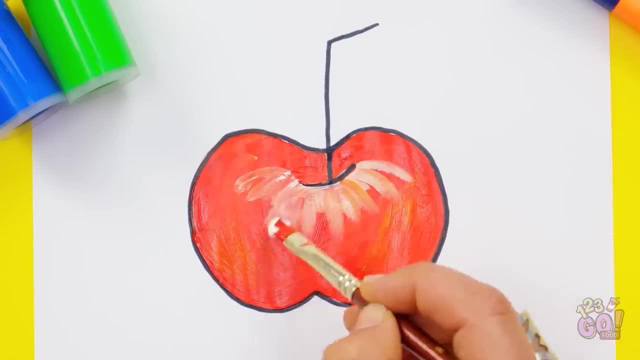 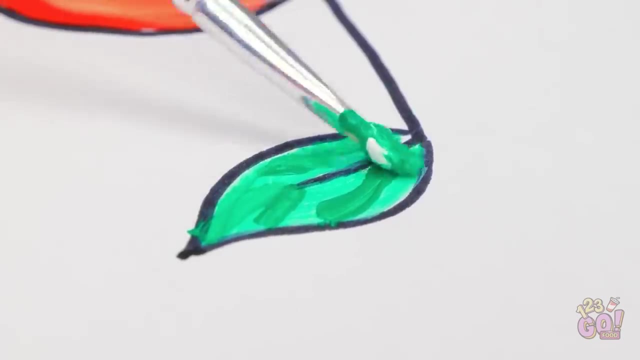 Especially not when you fill it in With just the right blending, this thing jumps off the page. Oop, Can't forget about the stem. Create a little shadowing And a few extra little details, And this thing looks good enough to eat. 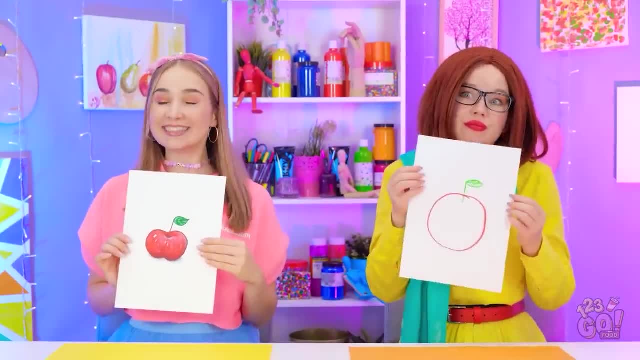 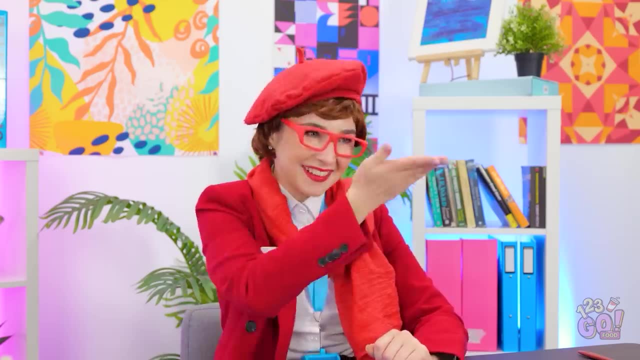 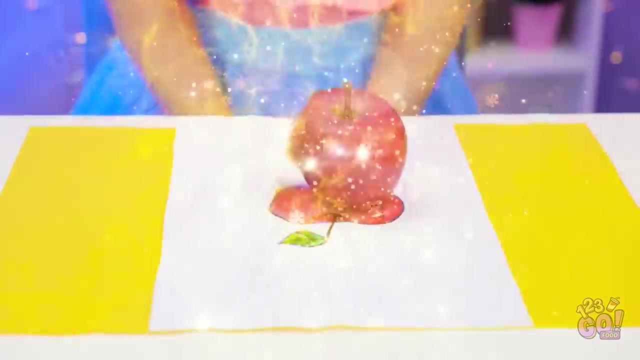 Don't you agree? Ta-da All finished Me too. How realistic And how… flat. Well, this is a no-brainer. Bravo, Annie, I won. Yes, I wish I had a real apple Me too. 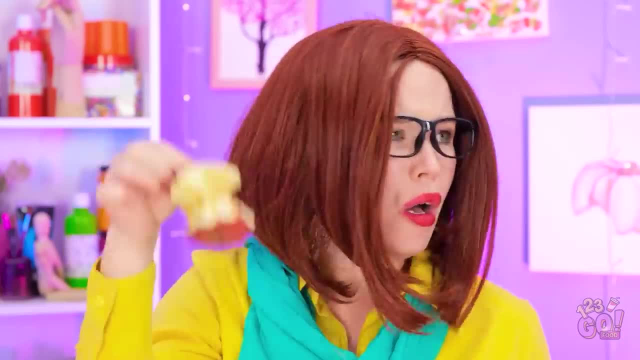 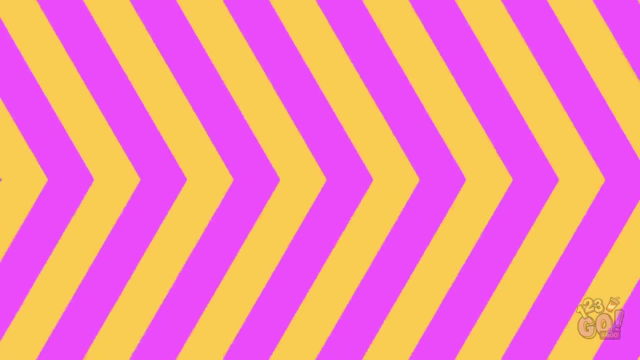 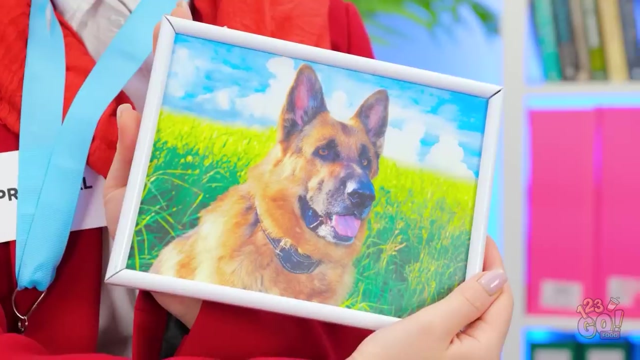 Ugh, Someone already chewed through this one. Ugh Hah, Luckily mine's fresh. Aw, my sweet, sweet good boy, So handsome In fact, why don't you two draw him Now? Oh, it's on. 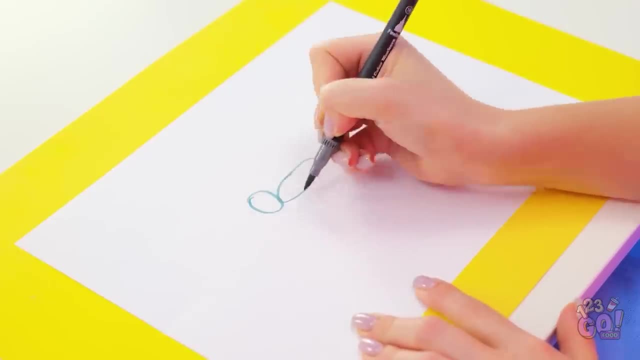 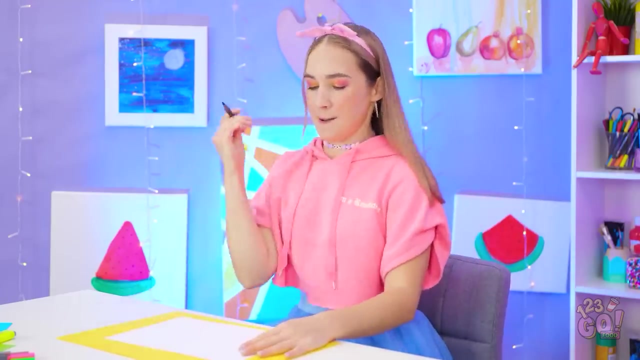 And I'm a doggy expert. It's just a head, body and four legs, But this looks a little dull, doesn't it? Ugh, Let me try this again. I think bigger's the way to go. Ugh, Still bad. 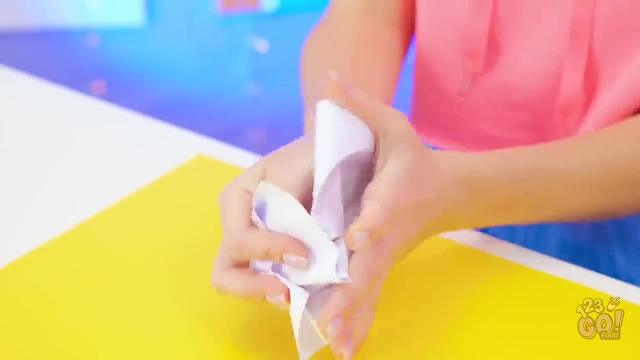 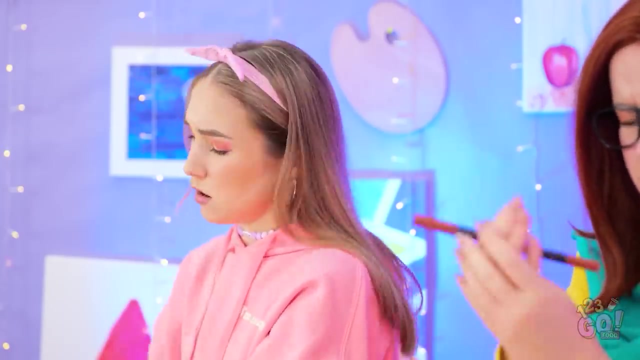 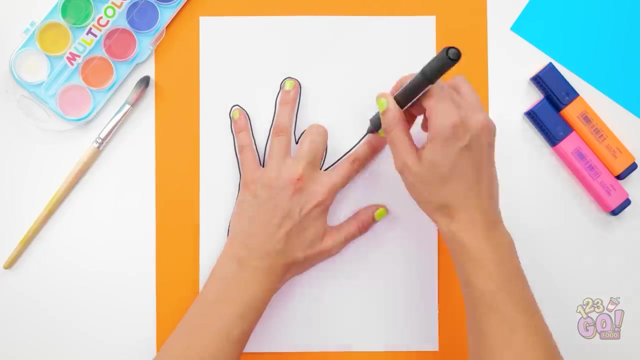 Hmph, Nope, Still awful. Gah, Ugh, Hey, Huh, What Calm down. Hey, I think I have an idea. I can use my hand as a guide, Because once I have the outline down, 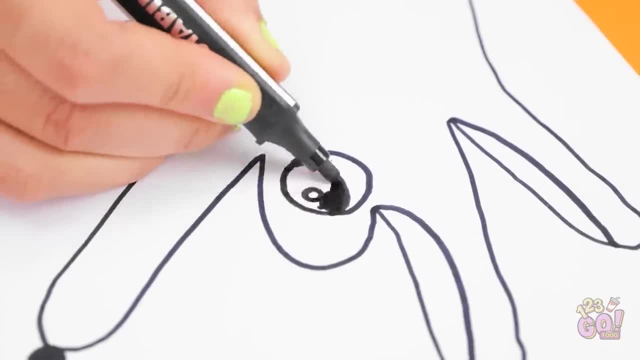 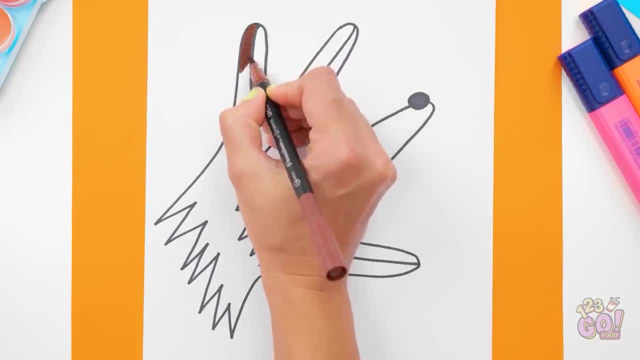 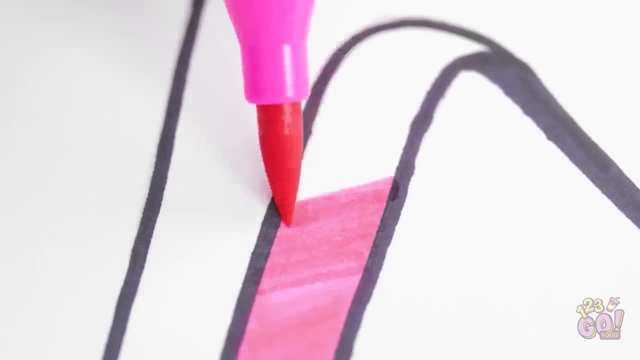 See, This is gonna be awesome. See, Now all that's left is some color, And this good boy is giving chocolate brown vibes. Can't forget that pink tongue, A doggy trademark. Ta-da, Like what you see. The resemblance is uncanny. 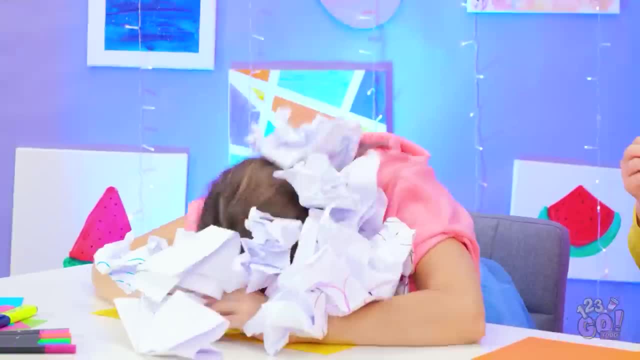 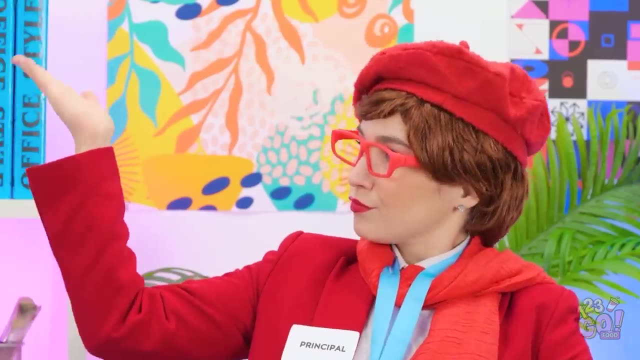 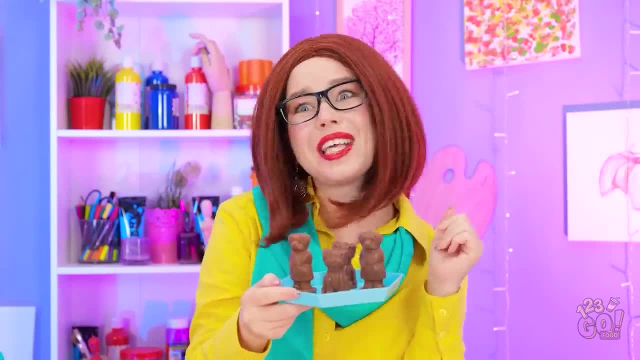 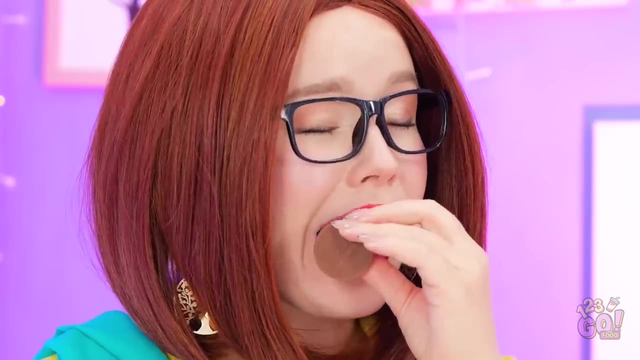 No drawing. That means you've won, Ms Emma. Ooh, these look delicious, Thank you, Chocolate doggies. I'm starting with this. one Looks good, Mmm. so creamy, No fair. Calm down, dear, just take one. 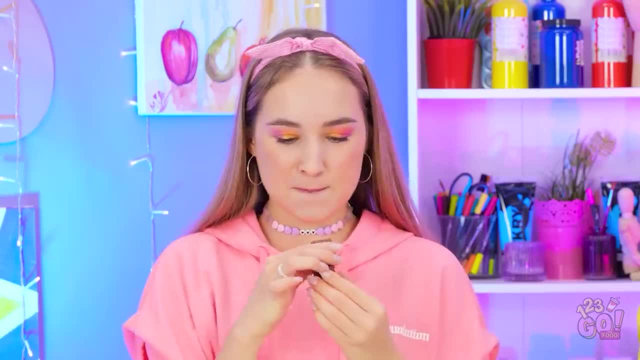 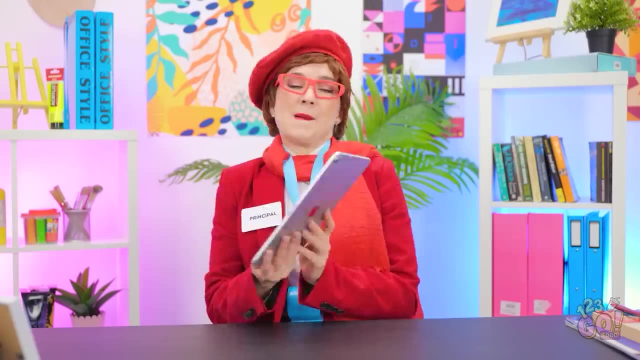 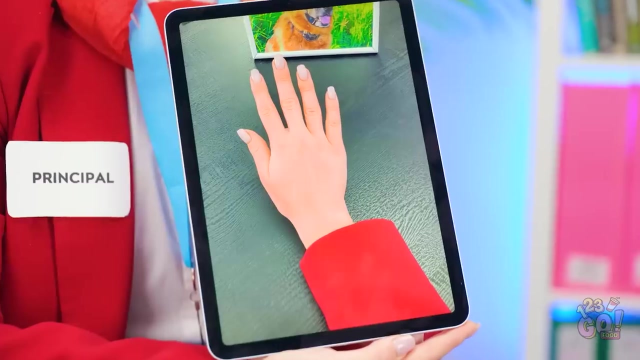 Oh, really, Thank you. Hmm, Of course, A little realism is in order, Ladies. Um… Hey, Oh, Sorry about that. Is that a hand we're drawing? Okay, fine, I have a plan, Let's see…. 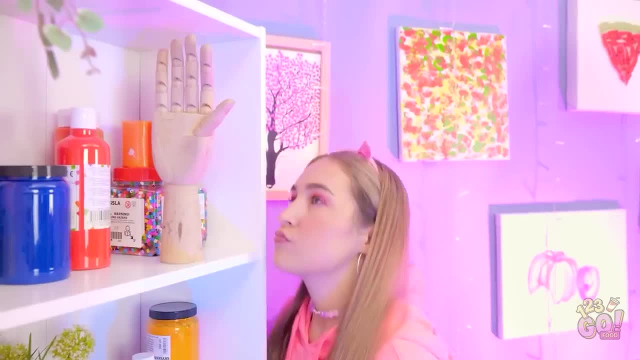 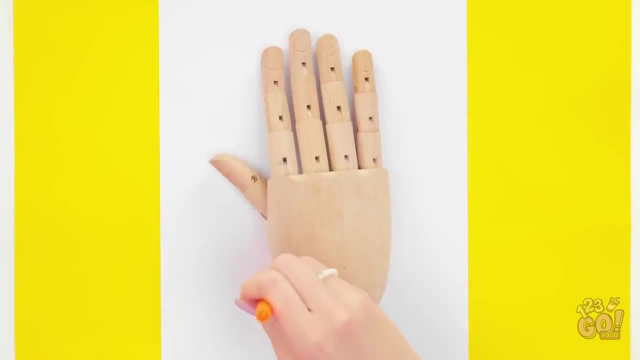 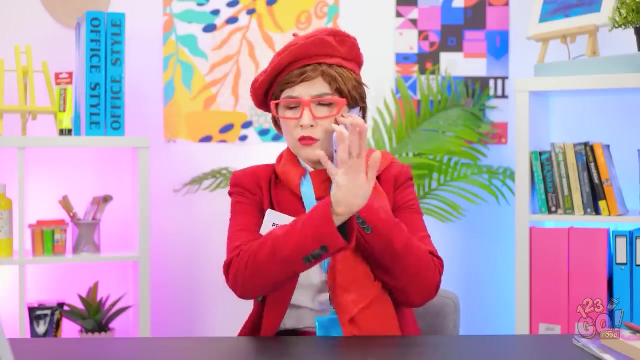 This hand could work, But this one is way better. Yep, Talk about lending a hand. All I have to do is trace this thing. I've got this round in the bag. Hey, look One moment… Seriously Okay, This thing's kind of fun. 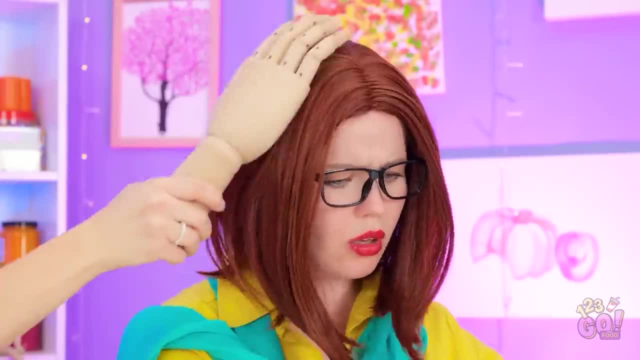 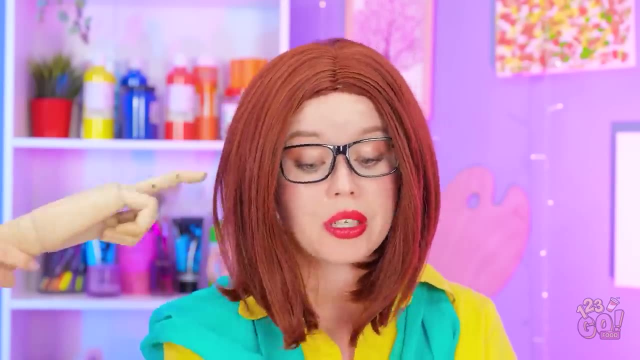 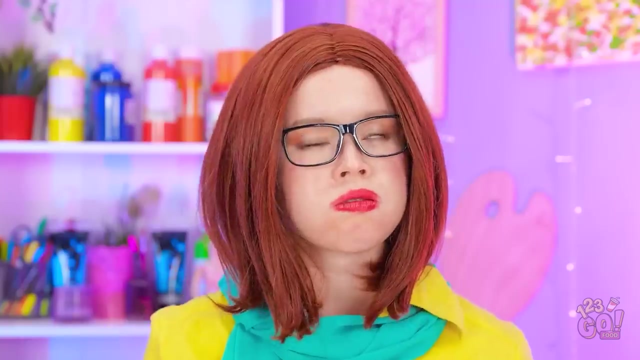 Actually… I know, Good girl, Huh, Annie. Huh. Well, that was odd. Got any wax in there? Huh, Knock it off. I'm trying to work here. Ugh, Wait, You know what This may come in handy. 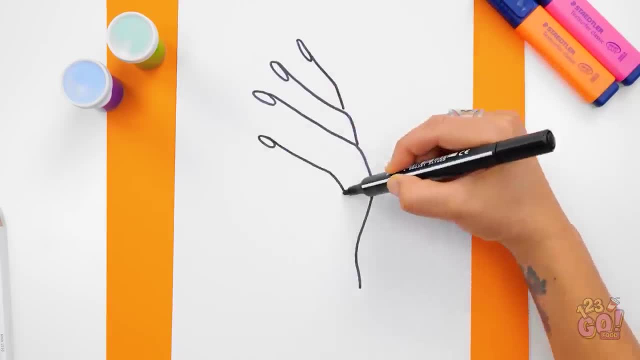 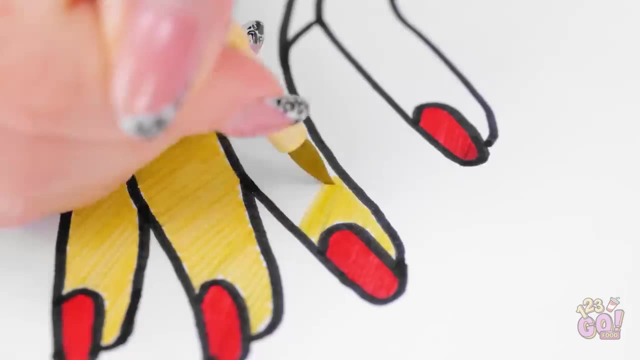 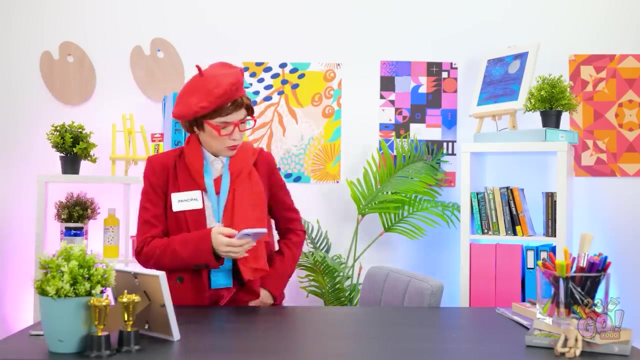 Art is all about inspiration, not copying. And those twisted fingers got my brain going. Can't go wrong with red nails. right, This thing is really coming together All finished. Where'd she go? Ugh, Anyway…, Hey, Hands up. 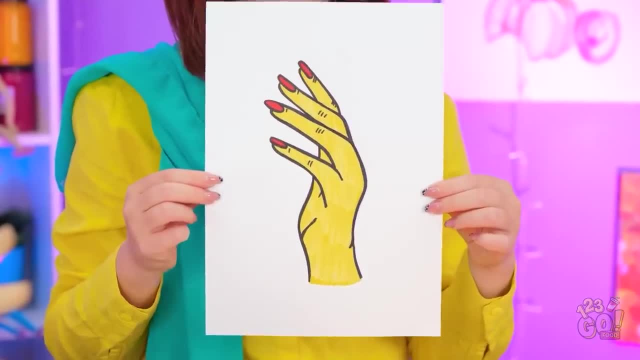 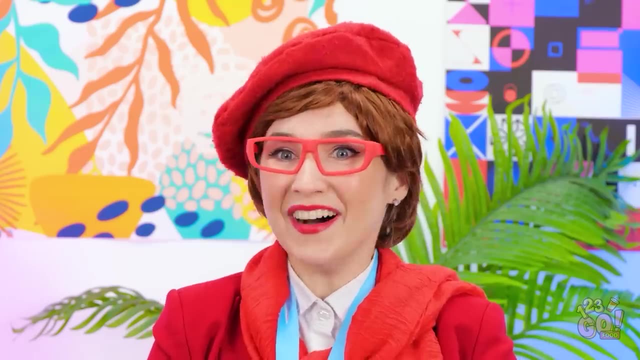 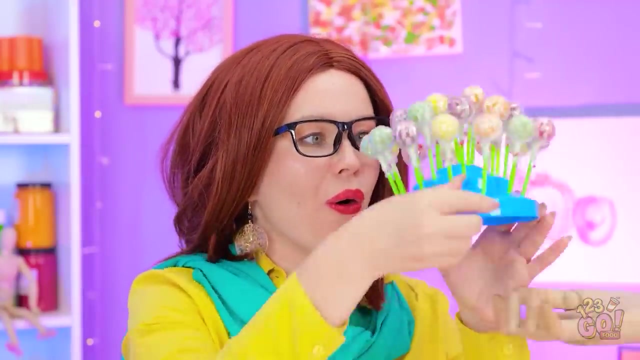 Okay, Whoa, How'd she manage that? Mine looks so lame next to hers. I'm so sorry, Meh. Oh, my word Stunning. Who's she waving in? Just my prize is all. And wow, this one's spectacular. 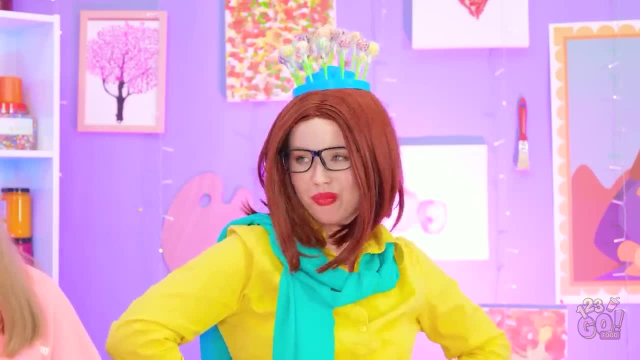 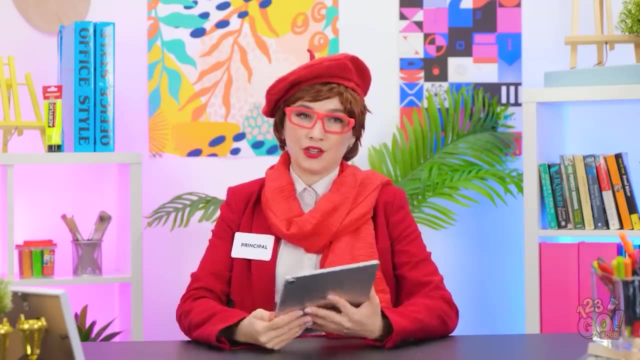 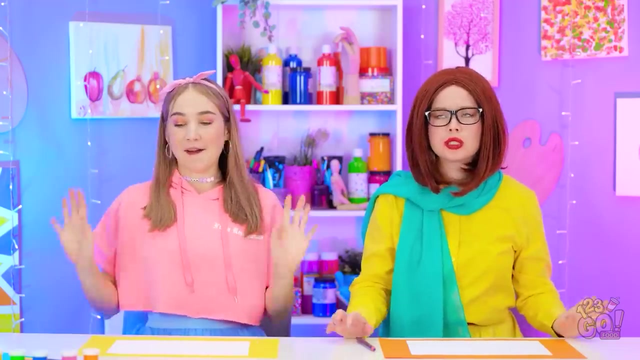 I'm the art queen Jealous. Good job, Don't even think about it. Howdy folks Think you can draw this. Now get going. Psh, This is gonna be a piece of cake. Oh, Oh, Pink's the name of the game this round. 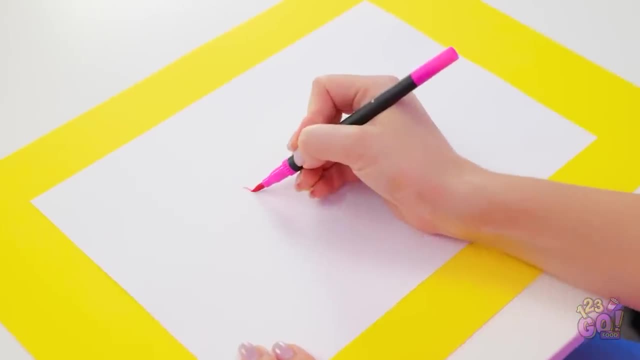 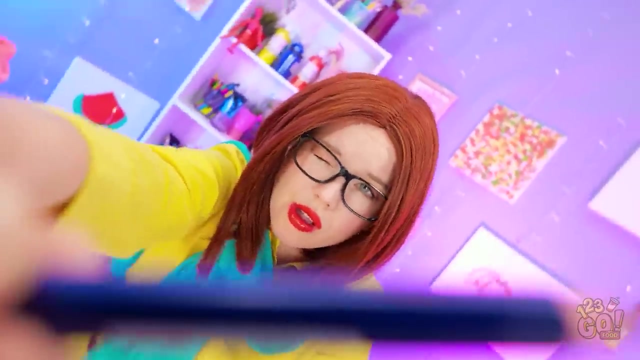 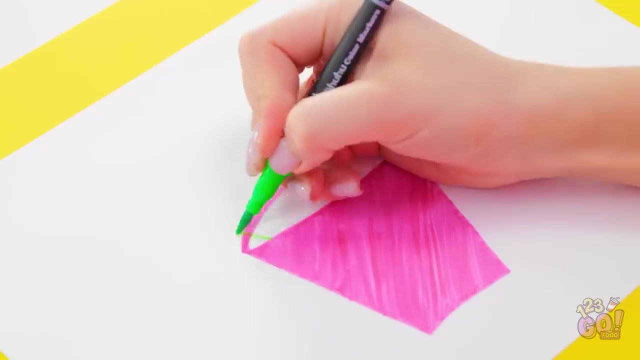 Oh yeah, First comes the paper cup. Bubblegum pink's my fave. Oh, She didn't even consider sizing. I'd say that's about five inches. Hmm, And now onto the yummiest part. So good, But maybe green was the wrong choice. 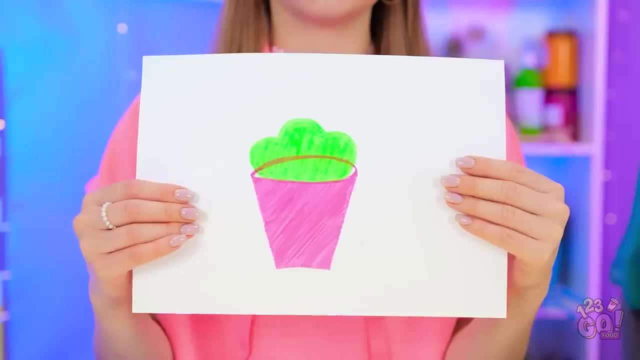 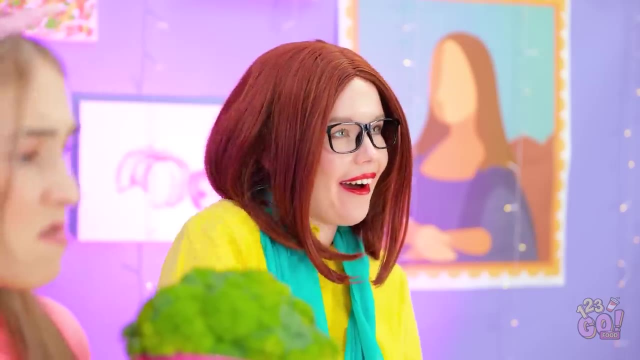 Yes, Yes, Is that supposed to be ice cream? Whoa, I didn't mean to draw this. You want a green right Amateur mistake. I say: the more realistic the better, Starting with the big creamy scoops. 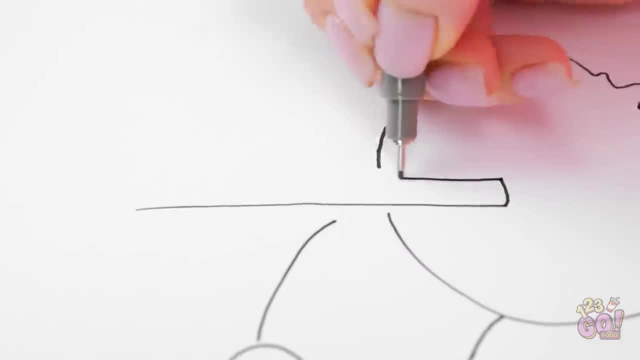 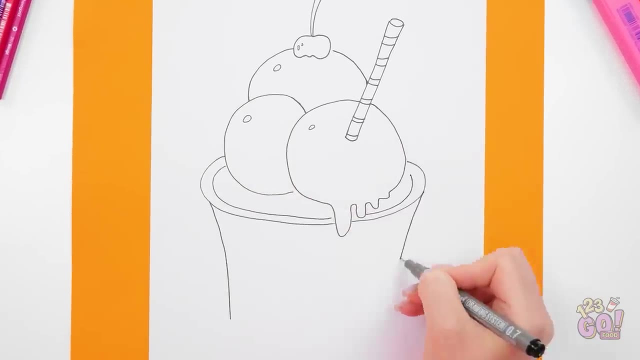 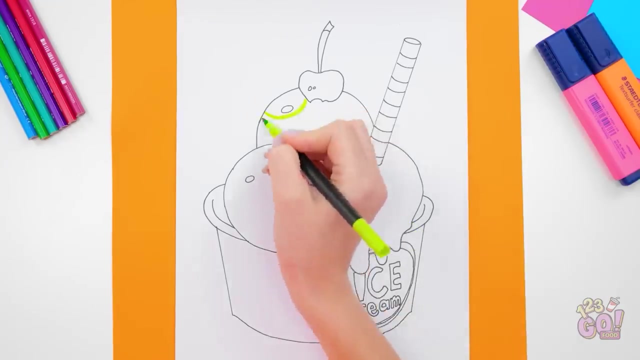 Color should always come second. You create a better foundation this way. See what I mean. You can't go wrong with all the little details. See Ice cream. It's written right on the cup, And now it's finally time for some color. 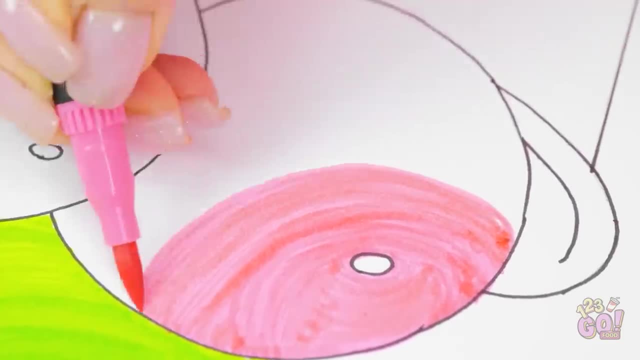 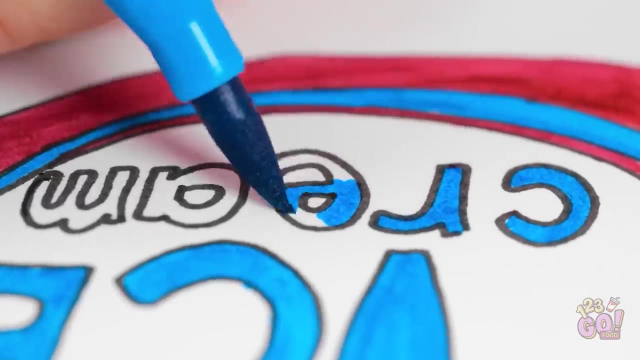 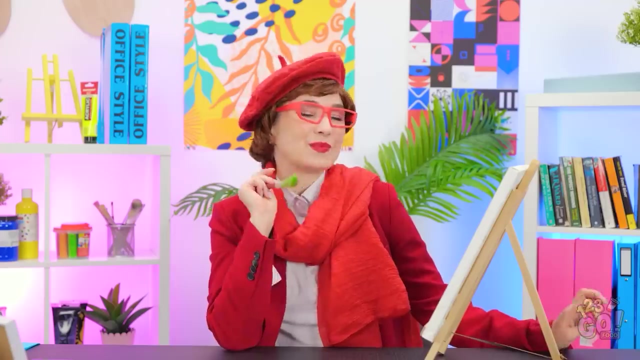 All this ice cream is making me hungry. That's what happens when you get real with what you're drawing. Almost done. Just a few more details here… And there I'm finished. Feast your eyes on this, Huh. Oh, let me see here…. 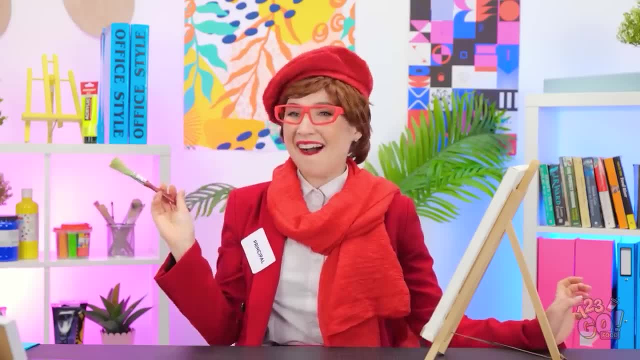 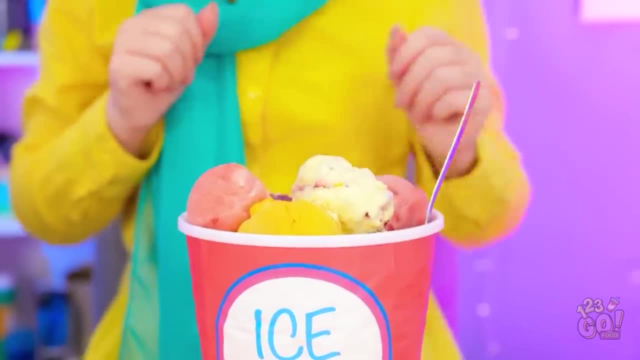 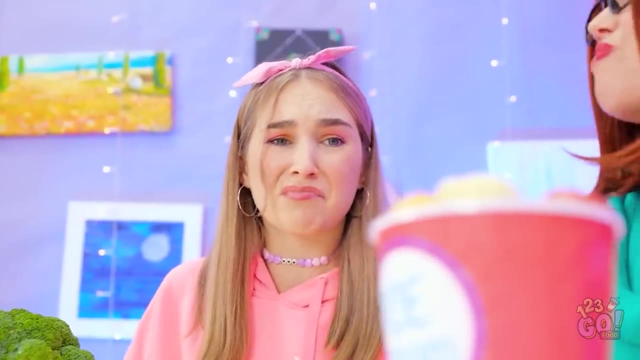 Oh, That's what I call a masterpiece Here. Yeah Whoa, It turned into a real bucket of ice cream. This may be the best prize, yet, Mmm Ugh, This is torture. I don't even like broccoli. 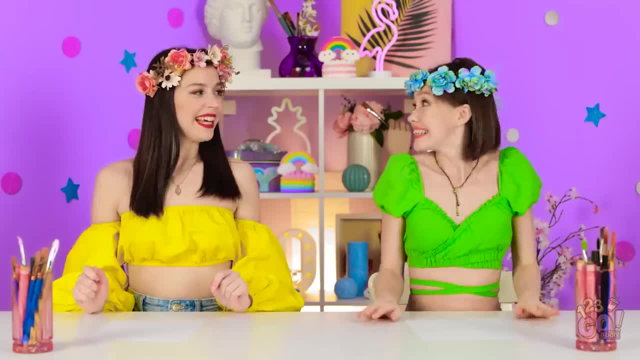 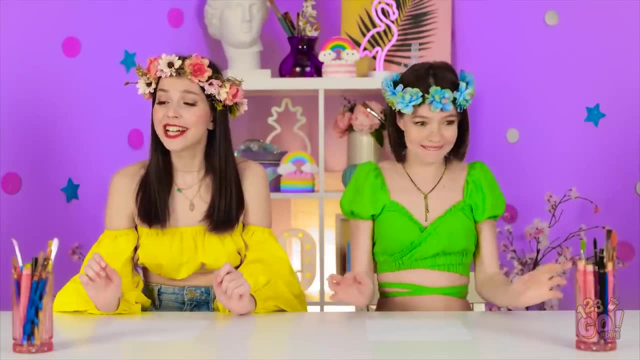 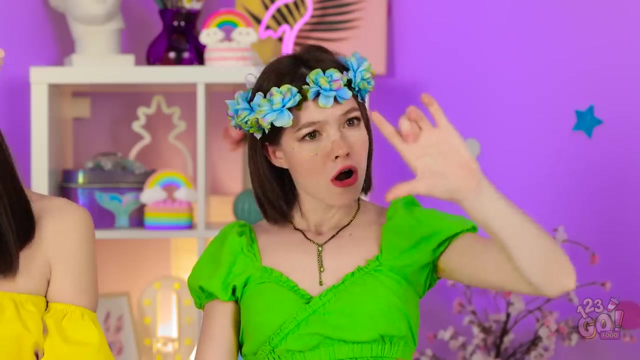 Ugh, It tastes like a tree. Okay, first challenge: I wonder what it is. Aww, What a cute puppy. Can we keep it? Okay, I can do this. Hmm, I've seen artists do this, No idea why, but it looks good. 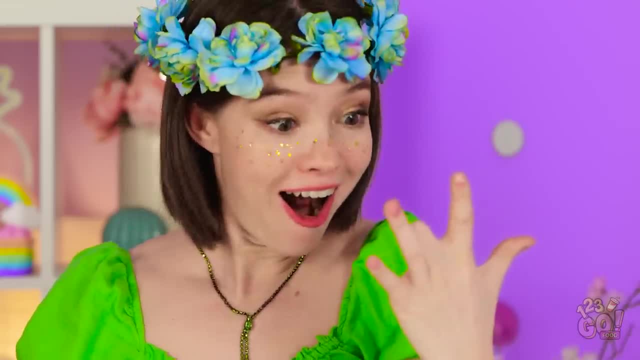 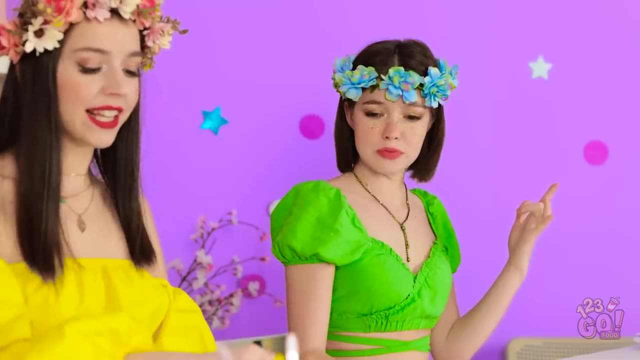 It's quite small for a puppy. Wait, I know what to do. Huh, I've got a hand too big deal. Ah, I get it. This is easy. I'll trace around my hand. What are you doing? 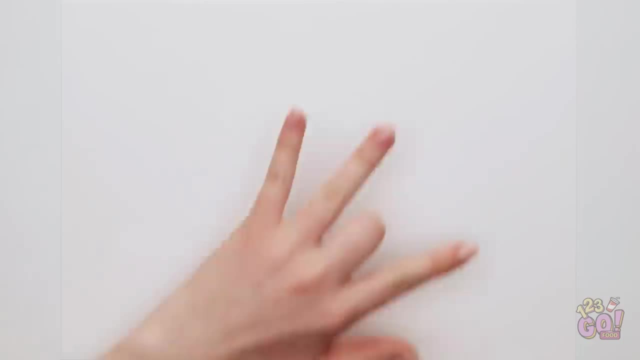 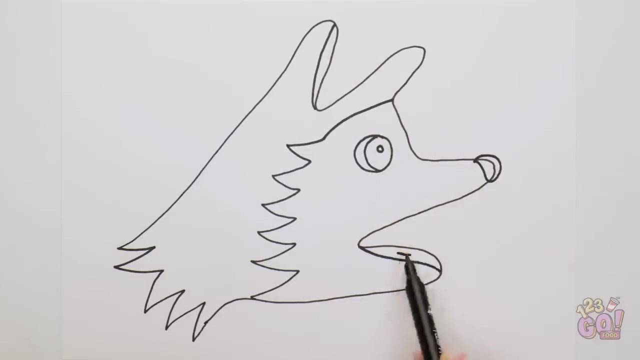 At least she's happy. I'll put my hand on the paper like this, Then draw around it Now to make it look like a dog: Some fur, Cute little eyes and a nose. I'll add some color. now This is turning out well. 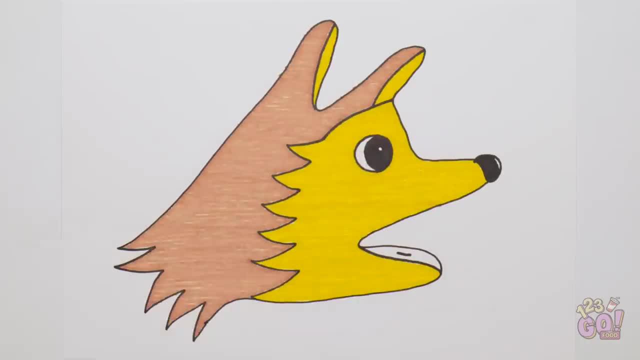 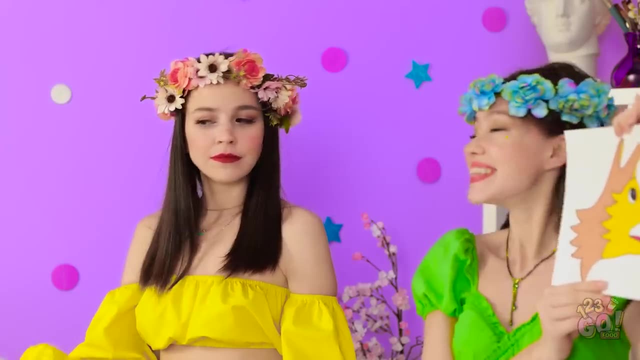 Gotta stay in the lines. Almost finished. There, He's so adorable. I'm proud of that. I'll call him lucky. That's actually quite good. I mean, I like mine, but… Wow, At least you tried. 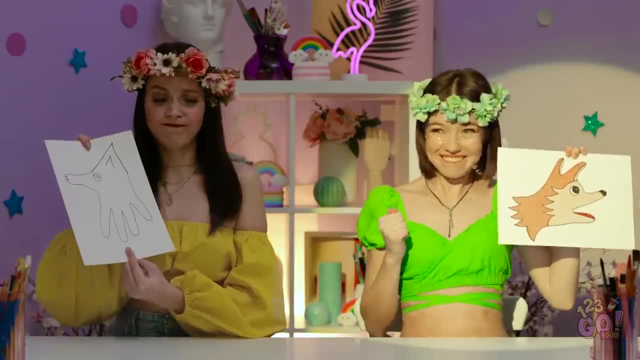 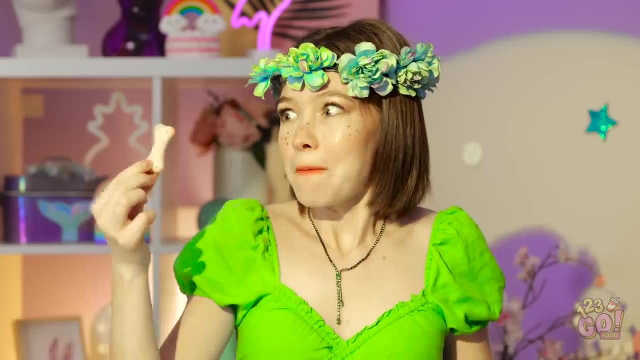 Who won? Yeah, Aww, Look, Look, Look, Something's happening. Biscuits, Yummy. It's shaped like a bone, Genius. I love the dog theme. I can't wait to try it. Hold on. 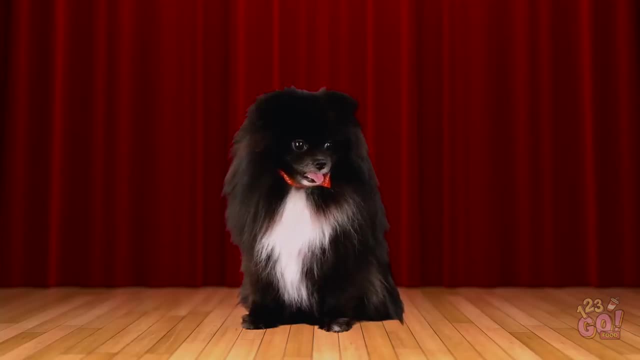 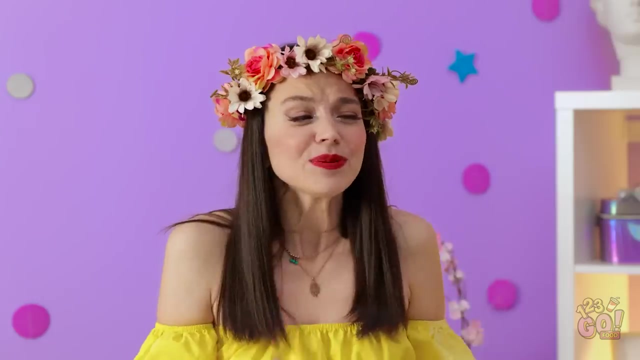 Biscuits: Bone Dog. Stop. They're not for you. Now, these taste great. I need the recipe. Ooh, I wish you hadn't done that. What's up These biscuits? They're for the puppy, Oh. 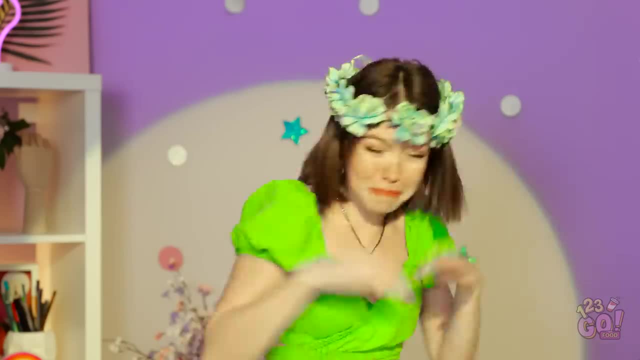 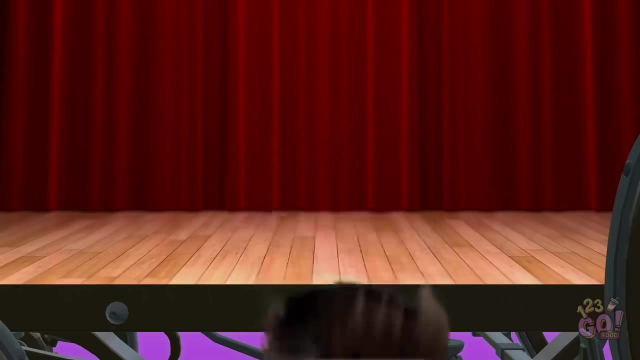 Oh, Oh, Oh, Oh, Oh. Could you not have told me that Sirs you right? Hey, come here, boy, We have goodies. Come on. Aww, Who's the best boy? You are, Yes, you are. 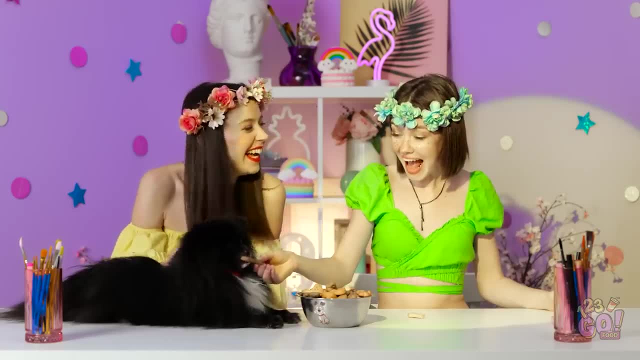 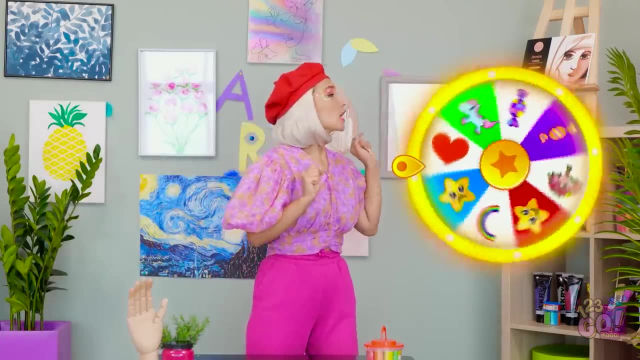 You must be hungry after all that posing. You're such a clever puppy. On you go, It's for you. La, la, la, la, la, Woo hoo, Oh, Oops, Sorry, class, What do we have this time? A star, 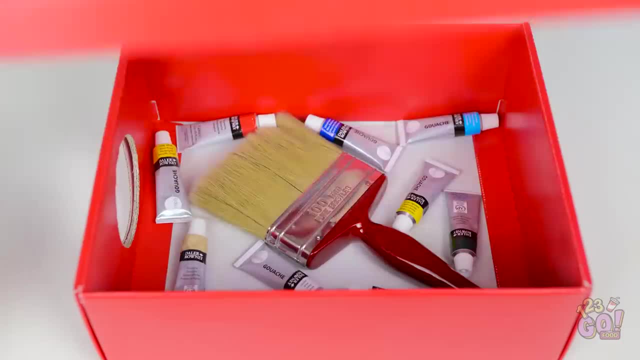 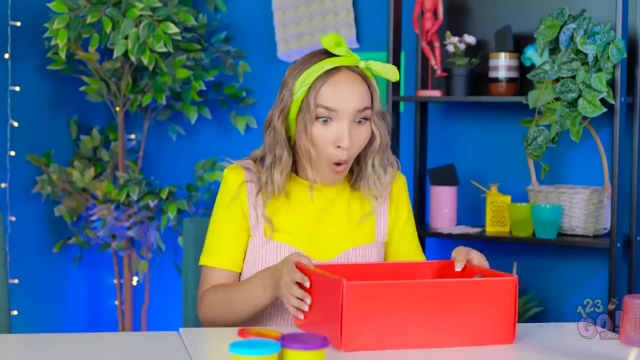 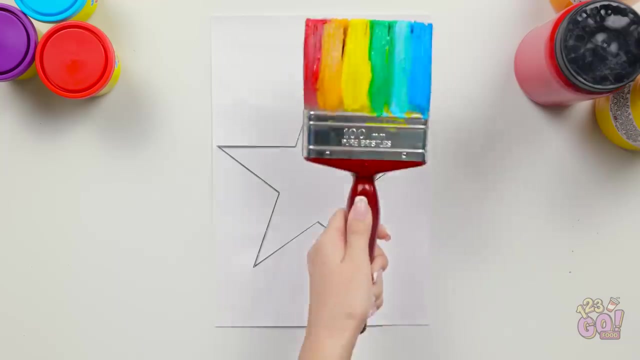 Begin. What's this? Paint supplies Whatever Polly can have it. Ooh, Look at this. Wow, This must be my lucky day. I'll place a template over the page And I've coated the brush in different paint. 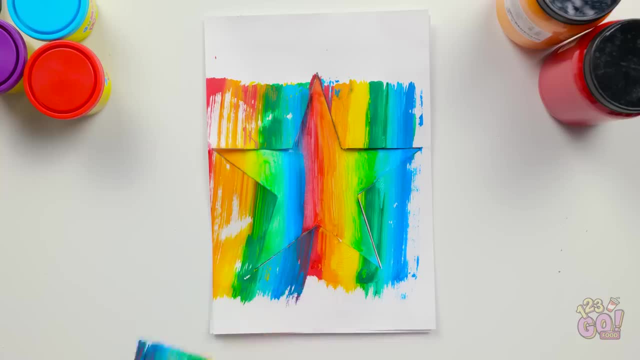 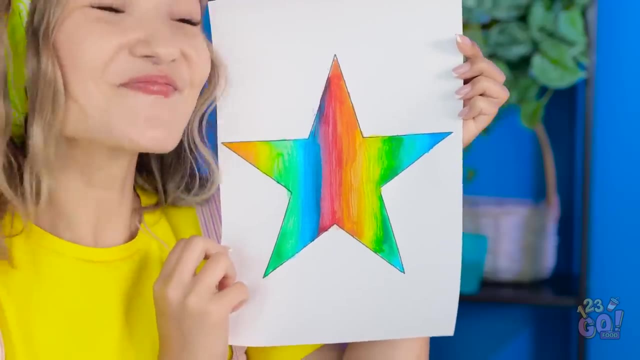 I'll paint over the template. It gives a great effect. Now I'll carefully remove the template. Wow, It's like a rainbow. I love it. That's the best you can do. I need to make a call. Hello, Yeah, I need some help. 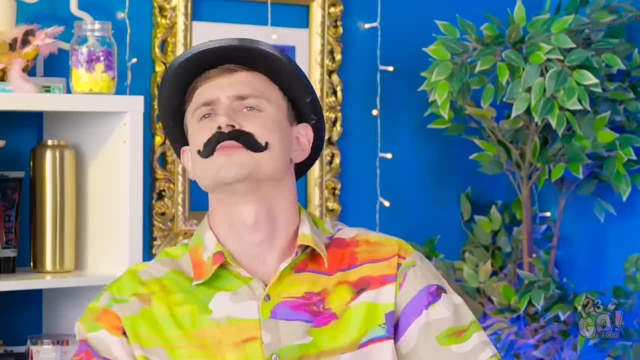 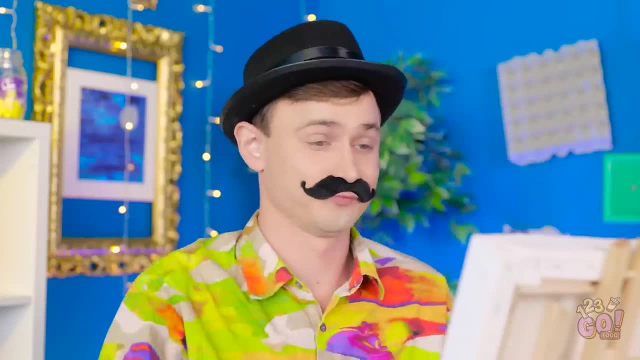 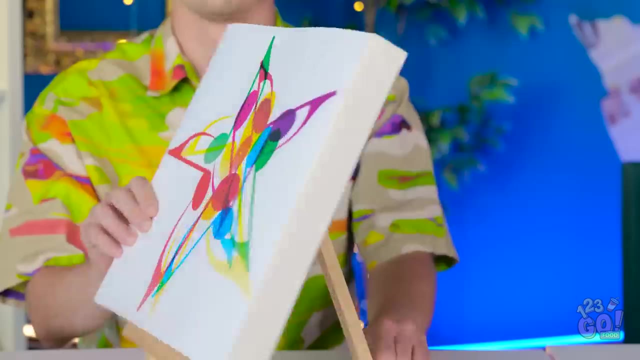 Ahem, What's going on here? Draw a star Easy. That's nothing to a professional like me. Watch and learn Something more challenging would be nice, but what can you do? And I'm done. You can applaud. now I know I'm talented. 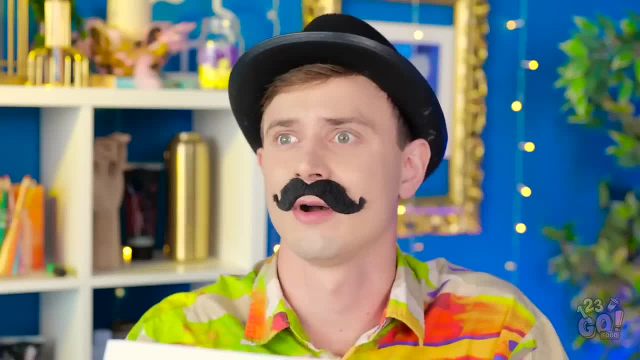 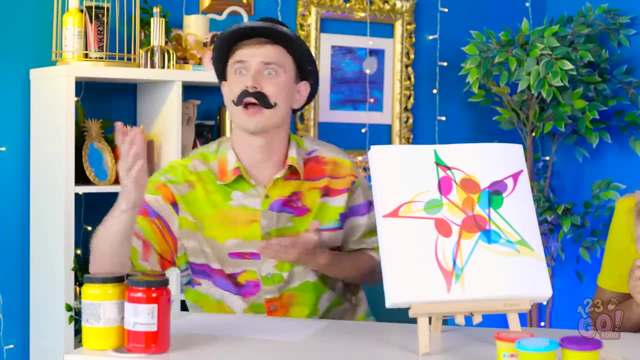 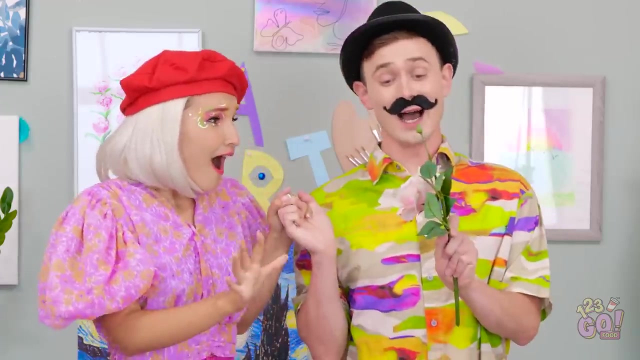 Oh, are you finished? Oh, My word, You are a work of art. You are my muse. Oh you, I could paint you every day. Uh, should I leave? I've never seen such beauty. This is for you. 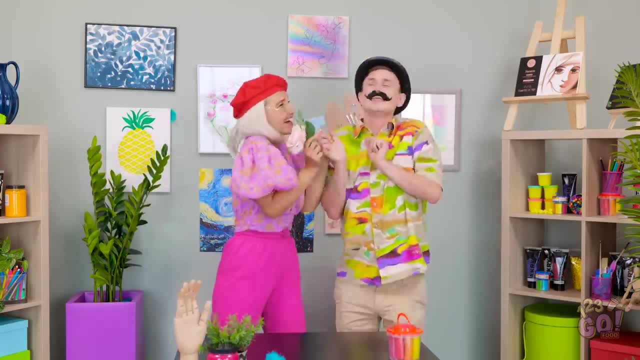 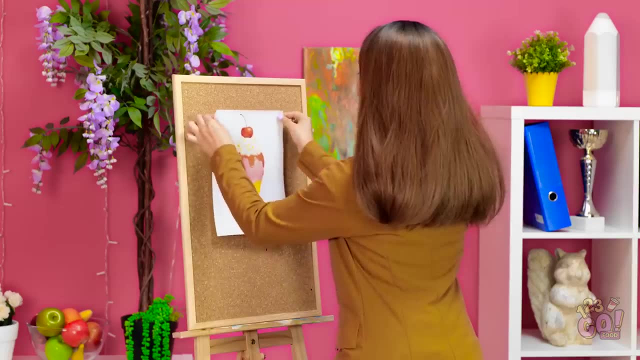 You're so romantic. I feel so inspired when I'm around you. Let's go. Hey, come back. My painting, Aww, All right, Next assignment is up, so pay attention. Hmm, An ice cream cone. huh, I can handle that. 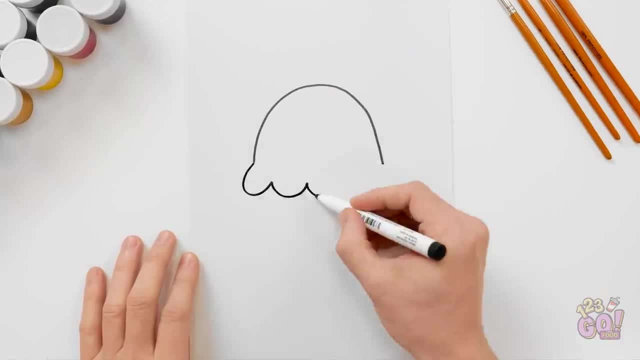 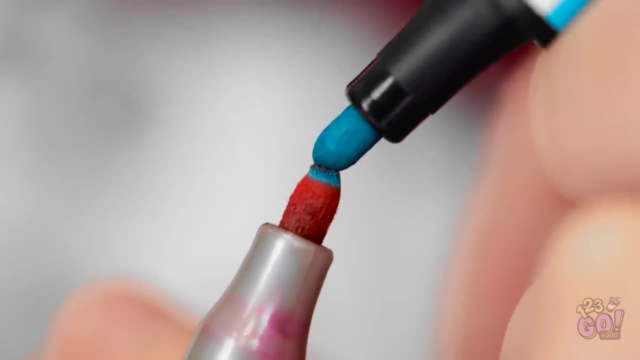 Time to use my artistic skills to get dry. Got the ice cream and cone done, Now to embellish it. There It's happy and cute. Next up, it's color time. I'm gonna fancify this, though. Okay, let's see if this works like I think it should. 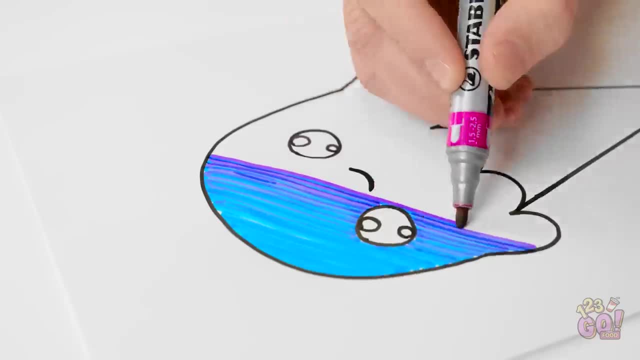 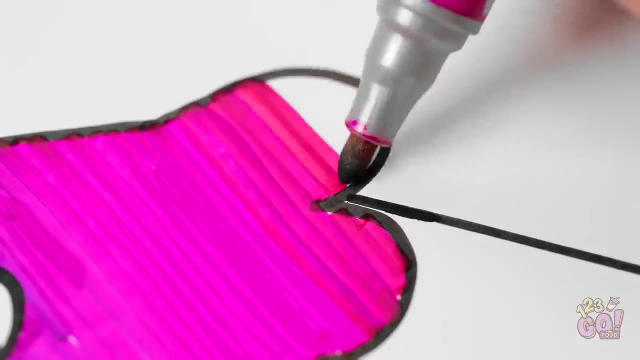 It's starting off blue, Now here comes the purple Gotta do around the eyes, And now it's finishing with pink, Just like I planned it. Excellent, Now that's what I call a great ice cream cone. Okay, better work on this cone too. 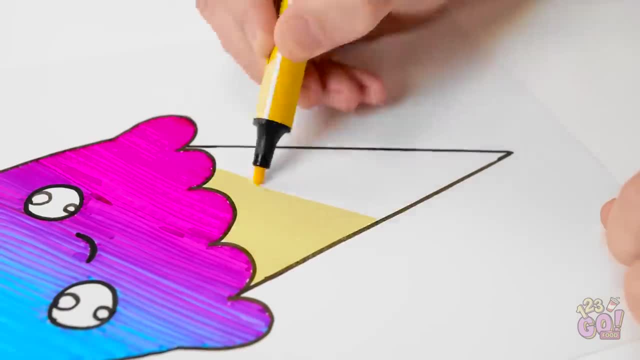 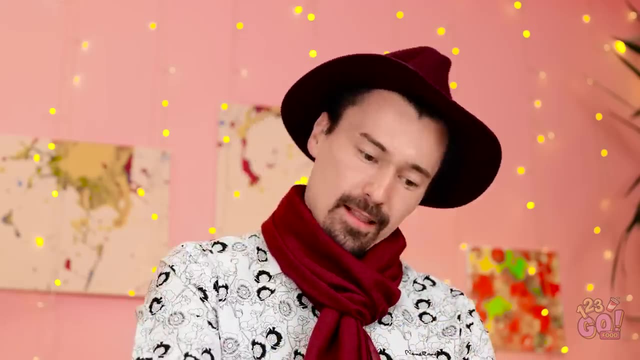 Can't leave that to be boring. This yellow will be a bold contrast, I think: Whoa, How the heck did he do that? It's amazing. Better check my point of view real quick. Yep, Good, I need to do something just as cool. 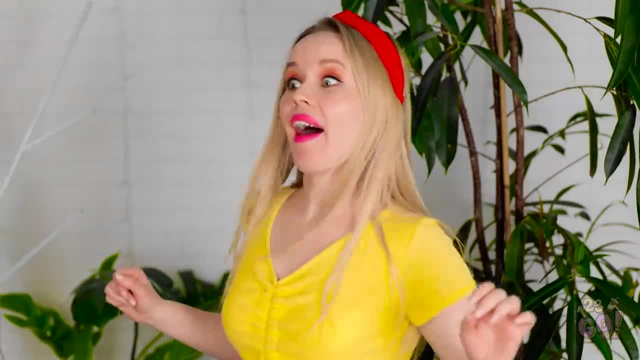 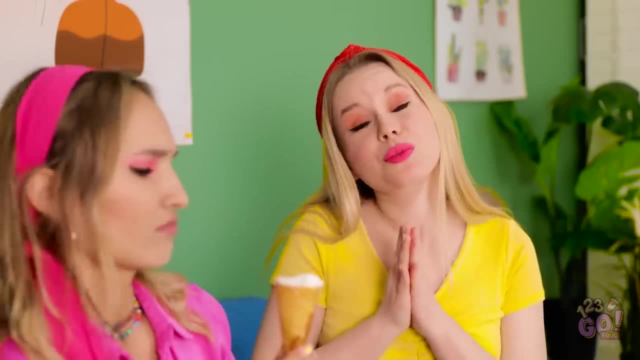 Let's see…. Oh, that's exactly what I need. Excuse me, Hi, Could I have yours please? Uh, I don't know you, so no way, But I really, really need it. What the heck It's mine. 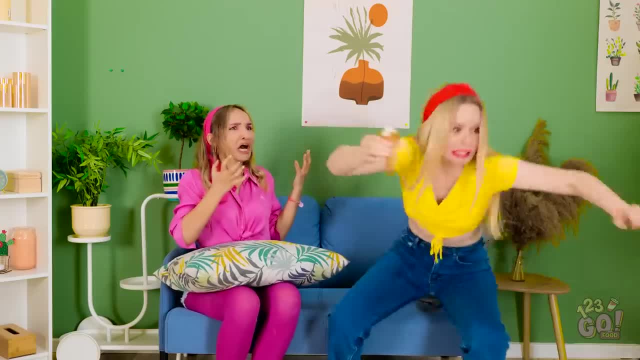 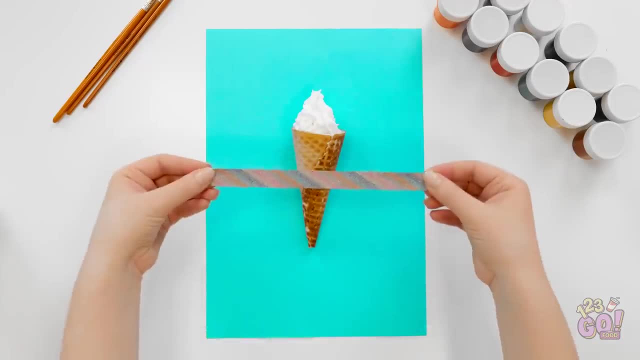 Let go and leave me alone. Oh Yoink, Sorry about that, I really am Phew. Okay, I'm back. I better get to work now. I'll use this pretty tape to hold the cone in place, Hmm. 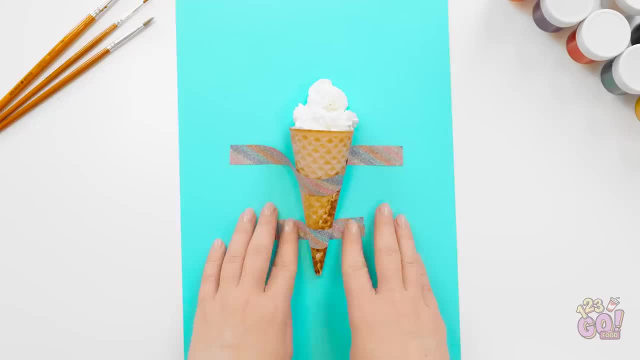 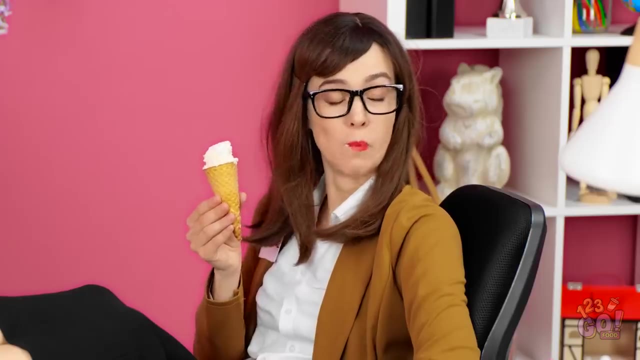 Looks like I might need a bit more, I'll add some down here. There we go. That should keep it nice and secure. Perfect, Ma'am, I'm ready to show you my art. Oh, already Exciting, Oh. 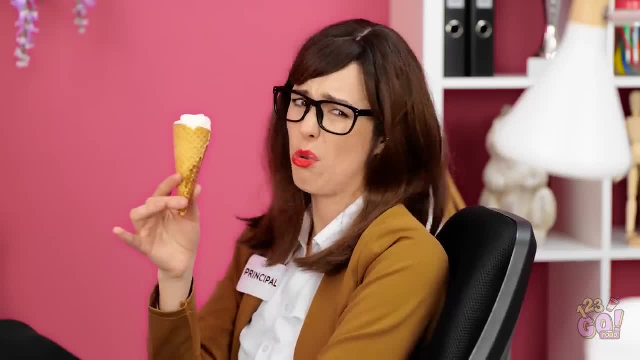 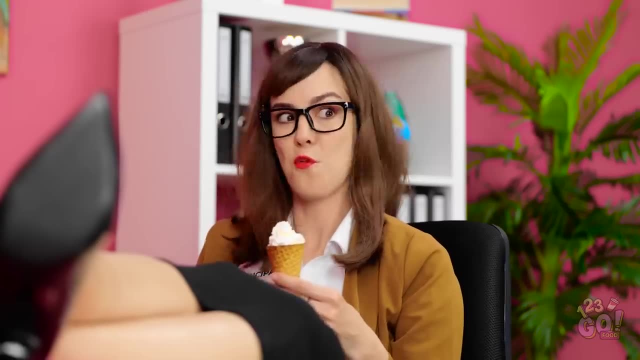 Does that really count as art? No, I'm not sure that it does. Hey, Show me what you've got. Oh, okay, then That's more like it. It's very cute and colorful. Here's your prize. Oh nice. 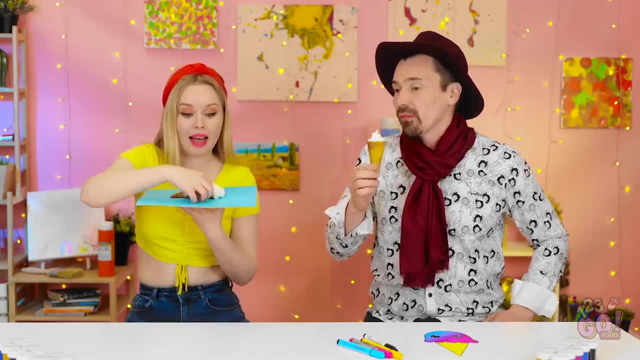 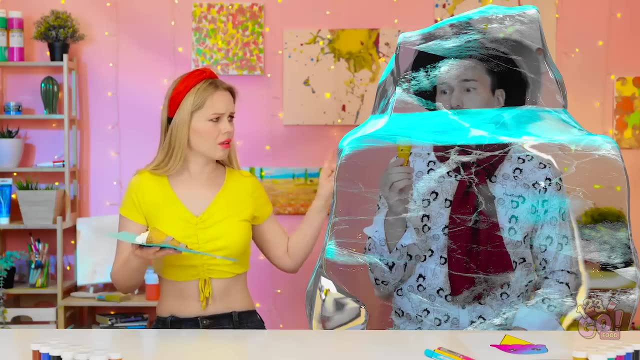 I was getting hungry too. I love ice cream. Oh, this one's pretty cold. Wait, what the heck Help, I'm frozen. Huh, What's going on with you? Oh, guess that ice cream was really cold. 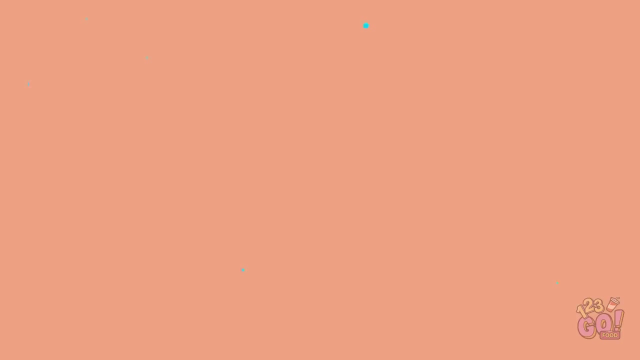 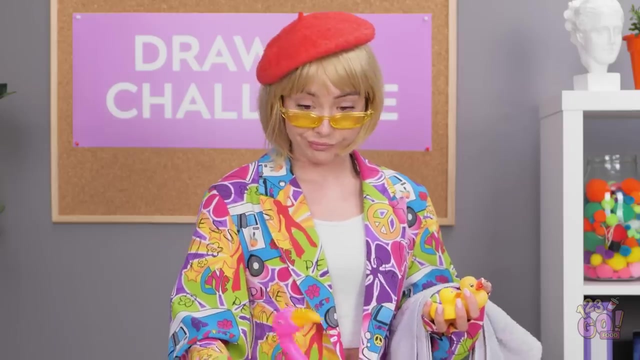 Oops, There he goes. Ouch, Hope he's okay. Uh, what the heck is going on with her now. I really don't get her. What's she doing with those towels? Hi, Yeah, we're still here, remember us. 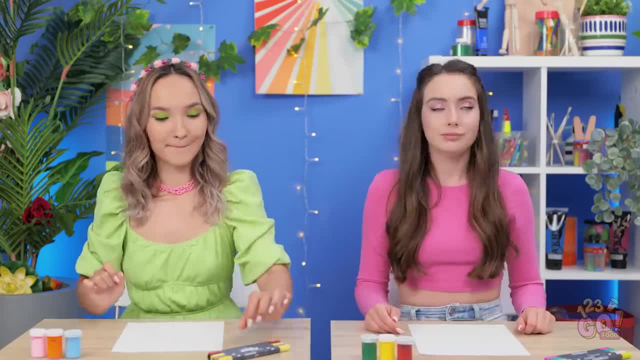 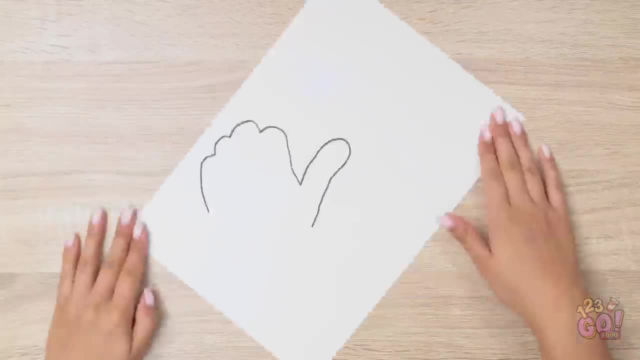 Well, okay, fine, then Here have this flamingo. Oh, a flamingo. Okay, this should be fun. I'm gonna go with my favorite method and trace my hand. Okay, good, Now to rotate my paper. This bird is gonna need a head, for sure. 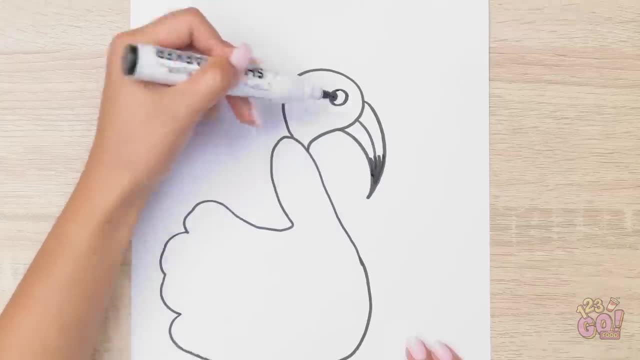 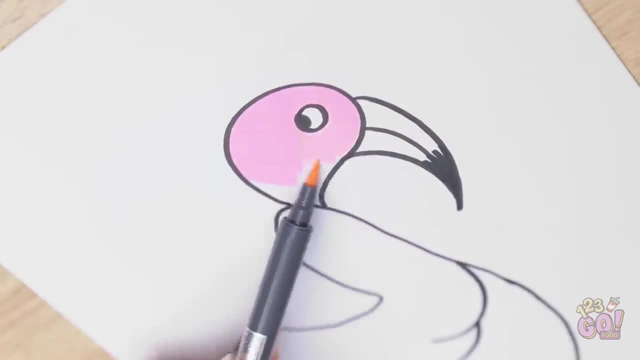 And then, of course, his big beak- Okay, eye is done. Now for the wings, And can't forget his long legs. Now for the color. Can't have a flamingo with some pink. He's gonna be so pretty when I'm done. 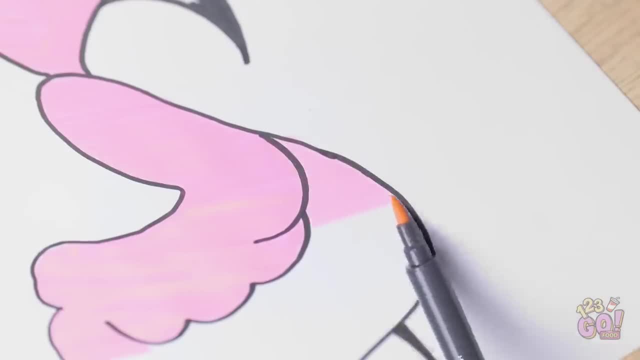 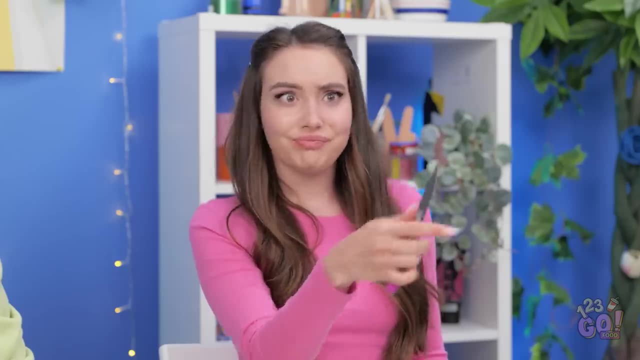 I just know it. Just keep coloring, just keep coloring. Just a little bit more and done. Let me see Gotta make sure to get the scale right. Eh, I'll just wing it. That was a pretty good pun, if I say so myself. 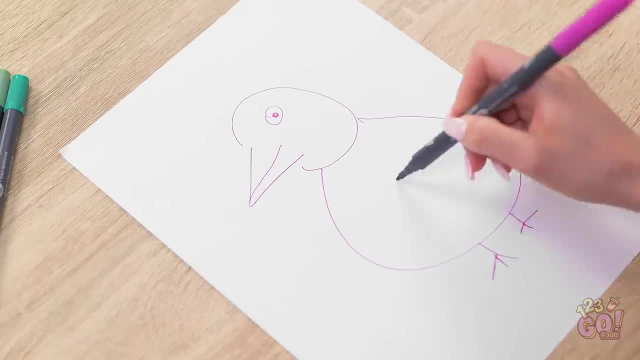 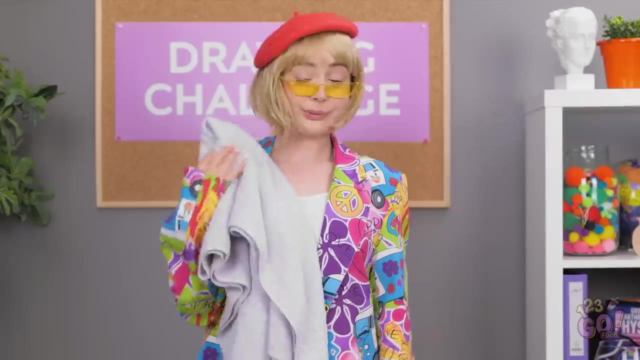 Okay, he looks something like this. I think, Okay, sure that's a flamingo, I guess. Phew, That refreshing bath was just what I needed. What do you got, Ew, What is that? Some sort of weird chicken? 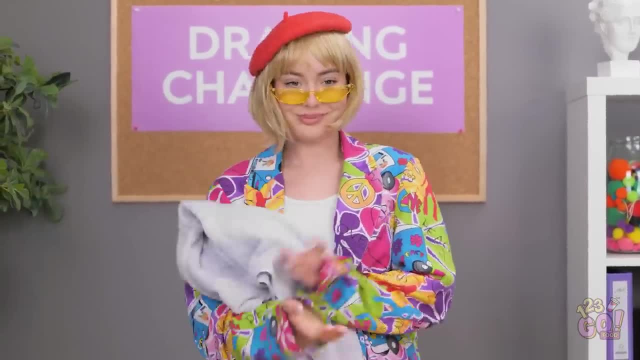 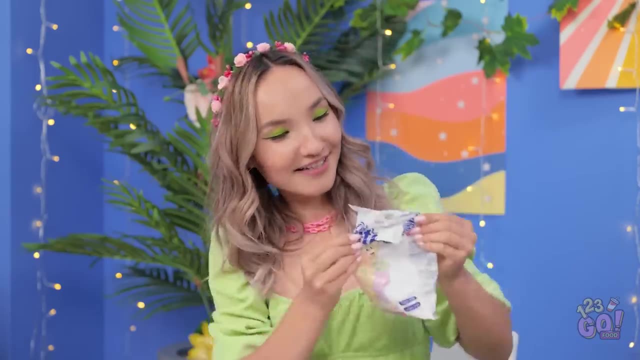 Aw, Yeah, sorry, I have to agree with her. Yours looks very nice, though. You win the flamingo challenge, Congrats. Yes, I won one all on my own. Listen, don't feel so sad, I'll share, of course. 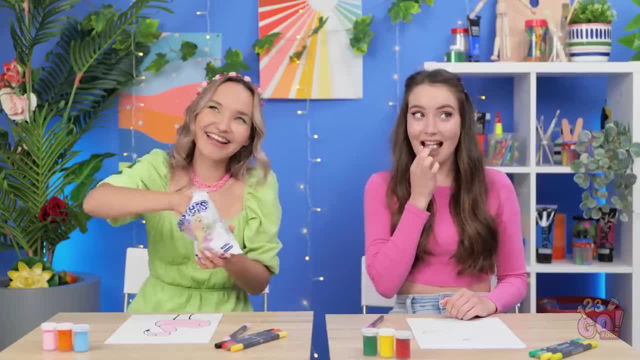 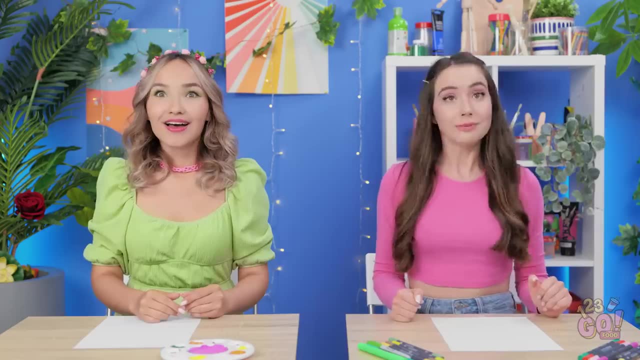 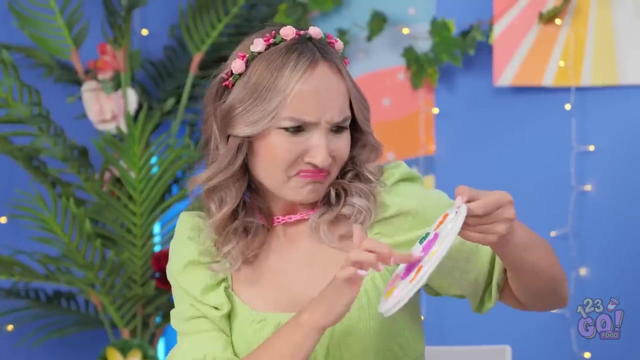 Here. Thanks, This does help me feel better. A rose, under any name, still smells as sweet. All right, yeah, It's flower drawing time. Huh, Oh no, My paint is totally tacky Shoot. What am I going to do now? 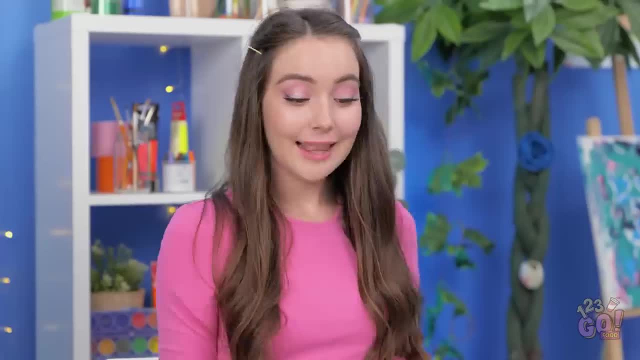 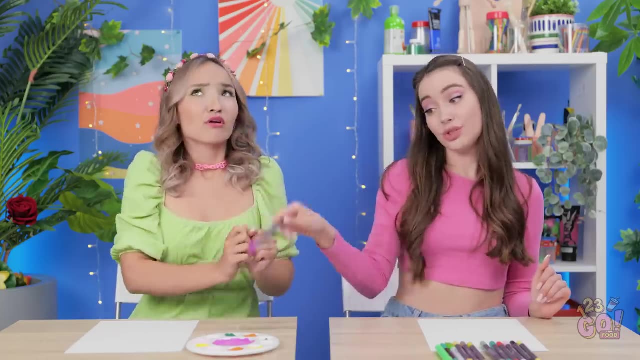 I need art supplies. Let's see Which color. should I start with? Pink, of course. No, you can't borrow this one. I need it Please. My paint is all tacky and too dry. I said: no, You'll have to figure something out on your own. 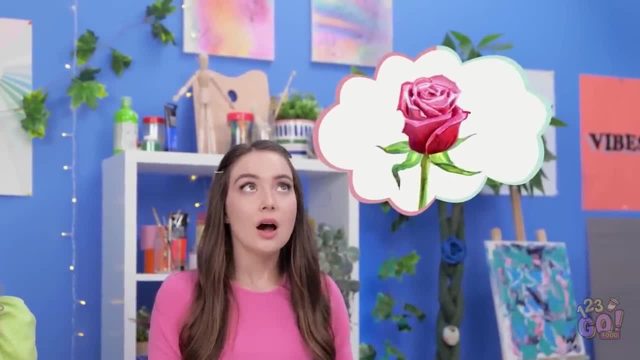 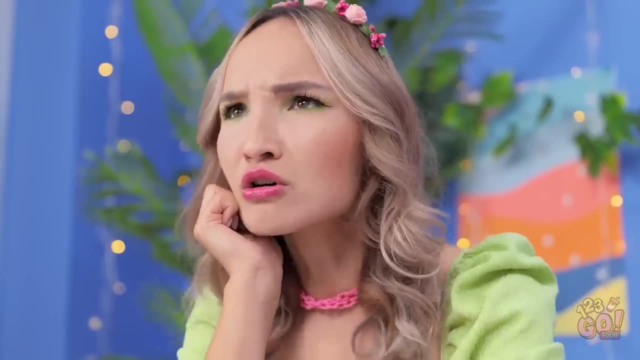 Now, how do I want to draw my rose? I want it to be beautiful. Okay, yeah, I think that'll work nicely. Ugh, I can't believe she wouldn't share with me. She's so mean. I'm getting myself all worked up over this. 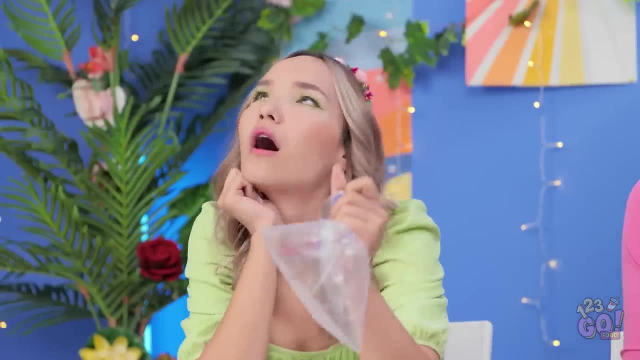 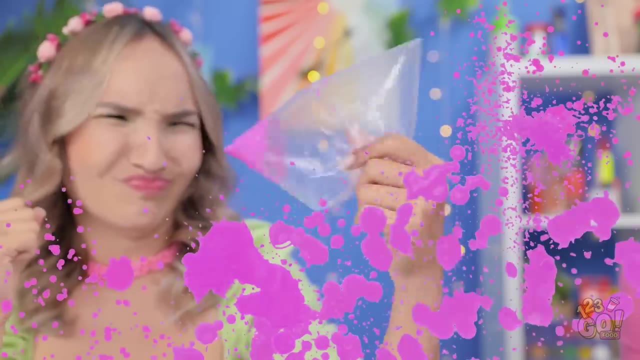 Ugh, I need to breathe. Whoa, I'm feeling a little lightheaded after that. Huh, What happened to my bag? Great, There's paint all over it. Get off paint, I said, get off. 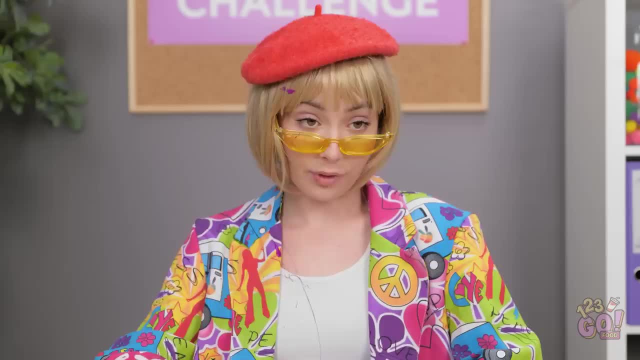 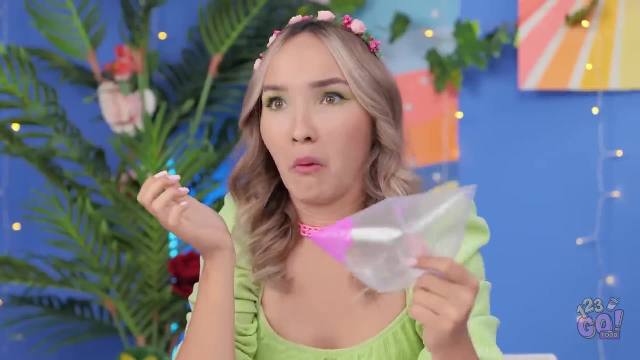 Ahem, What the? Keep your paint on your paper, please. Huh, Use the bag to apply the paint. Oh, Oh, okay, Got it. I guess I'll just dab it like she said. There's one, Maybe another one over here. 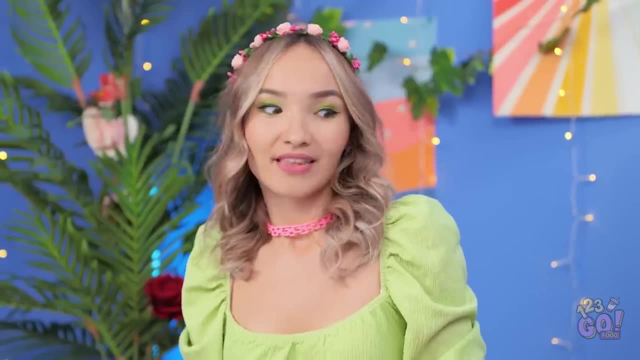 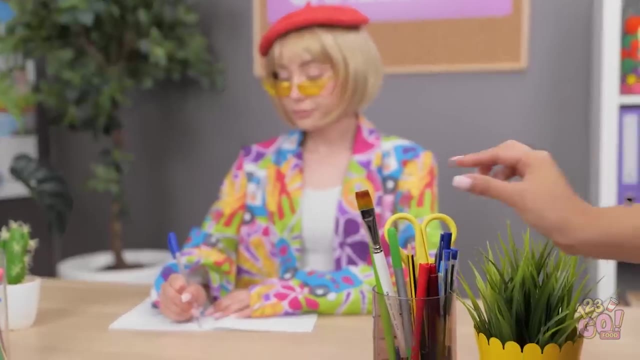 No way, These are turning out good. Great, Who knew? Let's see What else can I do. I know Where's she off to. Eh, doesn't matter, She can do what she wants. Just gonna borrow this. 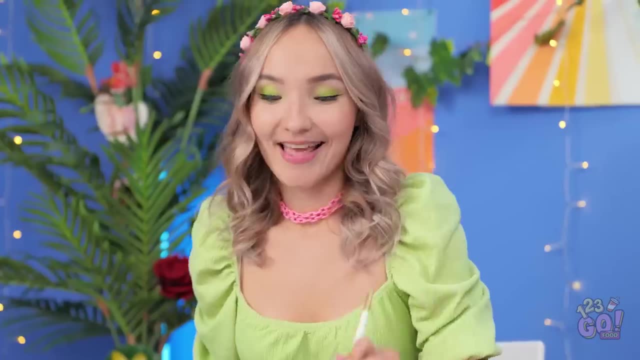 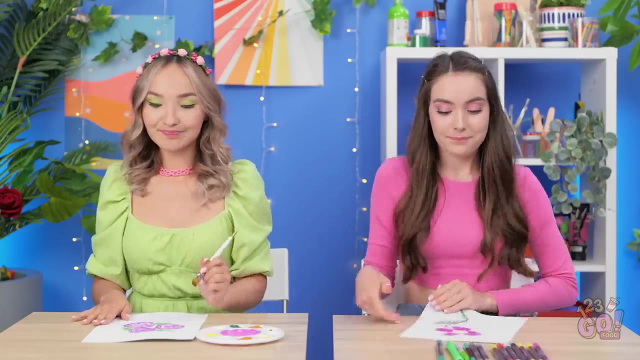 Yoink, Yes, Okay, I've got the paintbrush. Time to finish up my art. Can't have flowers without pretty leaves to go with them. Time's up. Let me see your rose artwork please. Okay, I'm ready. 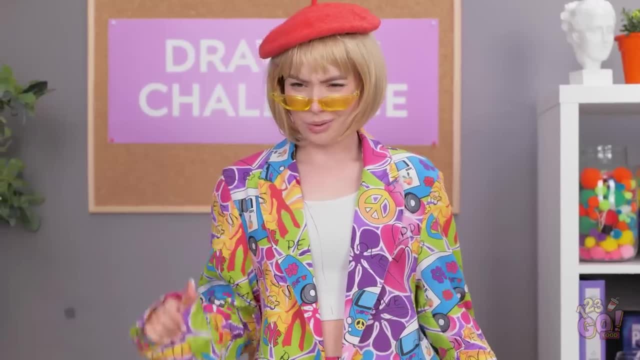 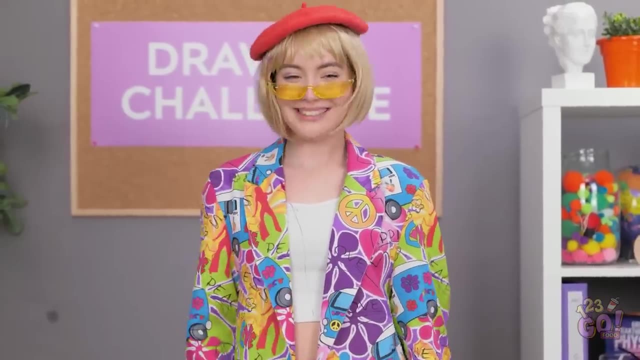 Here's my picture. Isn't it beautiful? I mean beauty's in the eye of the beholder, but no, it's not. Hers is, though. That's amazing It is, And that's why she's the winner for this round. 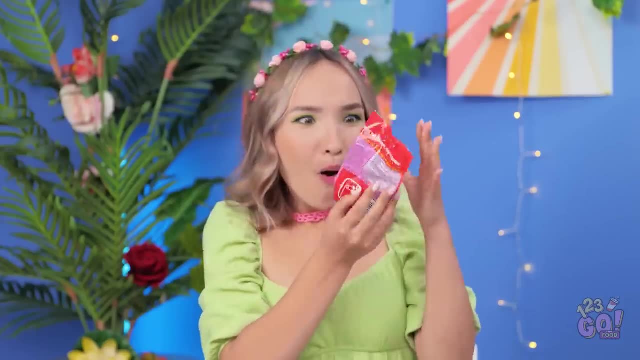 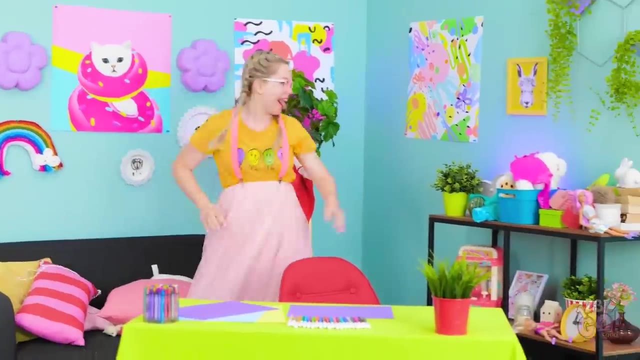 Yes, I won another one. I can't believe it. Ooh, Candy, My favorite, Look. Yes, Congratulations. Woo, This is fun. Ooh, What's this? Just look at her. Emma Put that down. 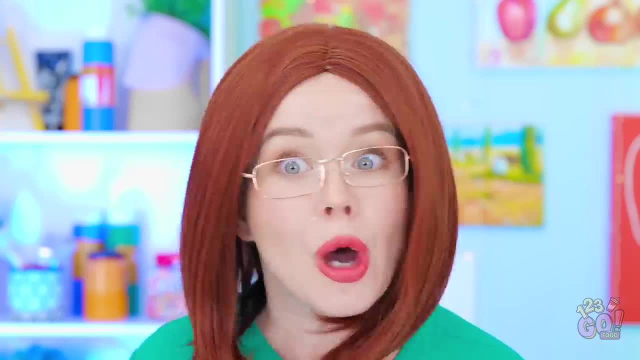 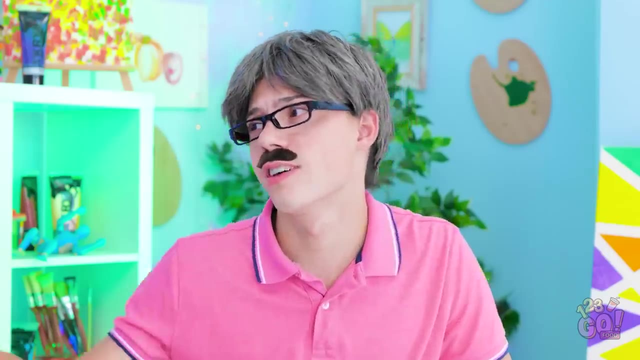 Nah-nah, Stop it right now. young lady, Are you listening to me? Uh-oh, Her eye is doing that weird twitching thing. That's trouble, Gah Ugh, Take it easy, Try this, Give me that. 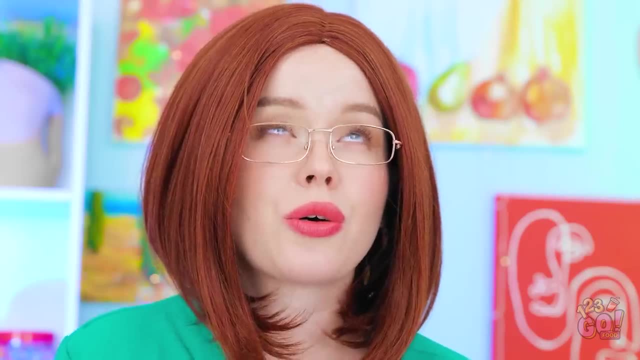 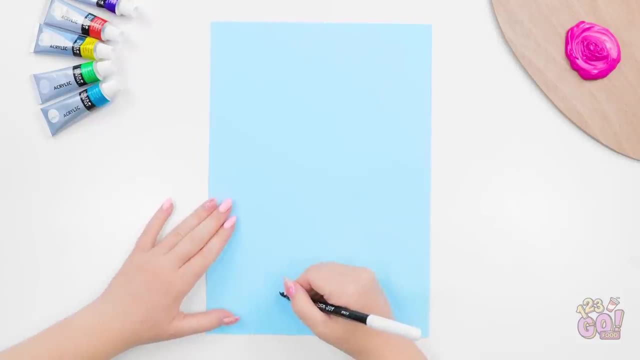 Ugh, I can feel the tension melting away. Ah, that's better. You just get me, dear. Wait, I think I can use this. I'll start by drawing a tree. You gotta love nature. This black pen is perfect for the branches and trunk. 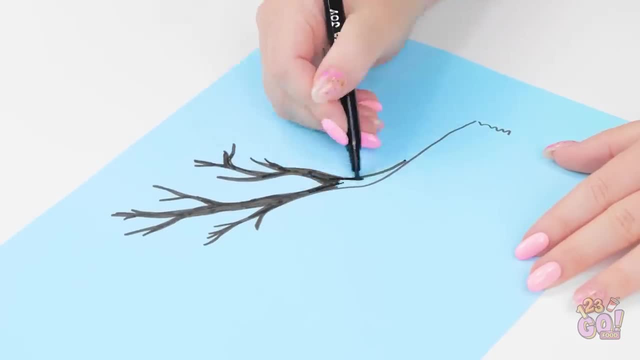 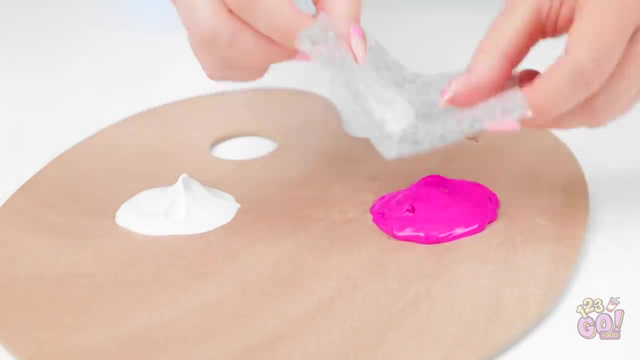 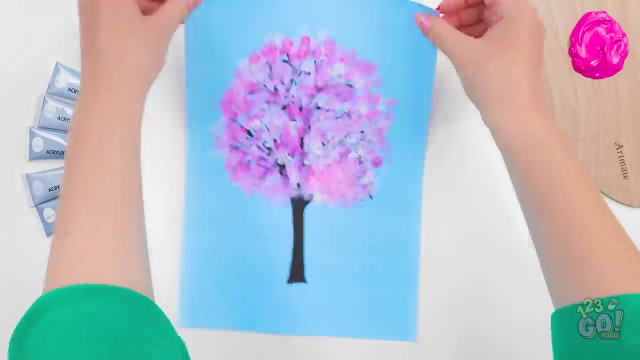 That looks good. Now I'll take a small square of bubble wrap and dip it in paint. I'll mix the pink and white. I'll dab it over the drawing. It gives the impression of leaves. It's a beautiful blossom tree, Do you like it, Emma? 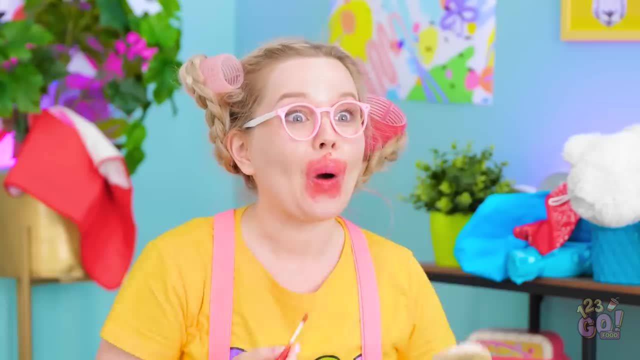 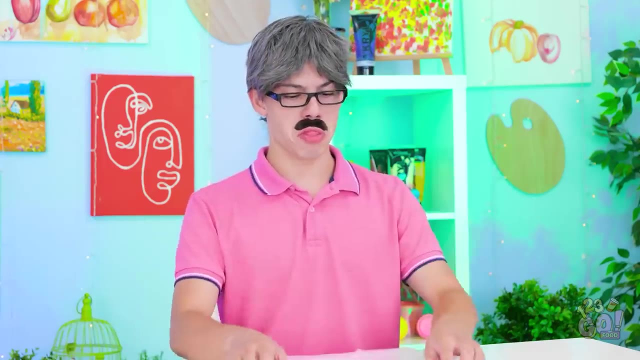 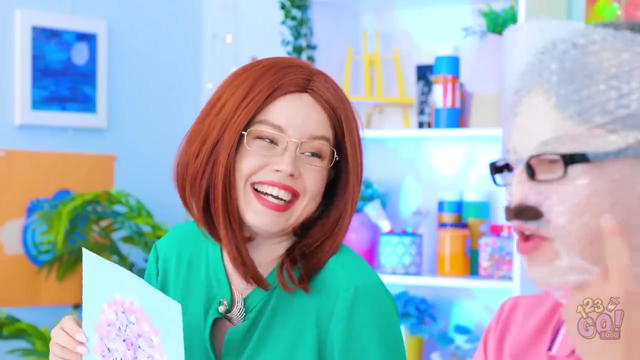 Oops, Silly me. Wow, Mom, It's amazing. Hey, Maybe I can use this too. I know what to do. How do I look? No one say better looking, I'm a work of art. Are you for real?